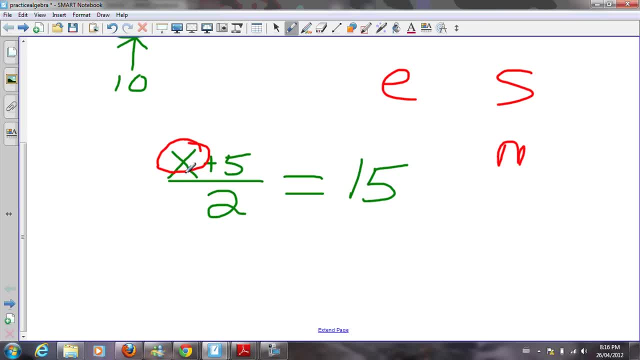 figure out how are we going to get this letter all by itself on one side and all of the numbers on the other side. So we're going to do a few examples with that and we're going to follow two basic steps in order to do it. So here's one of the sheets that was 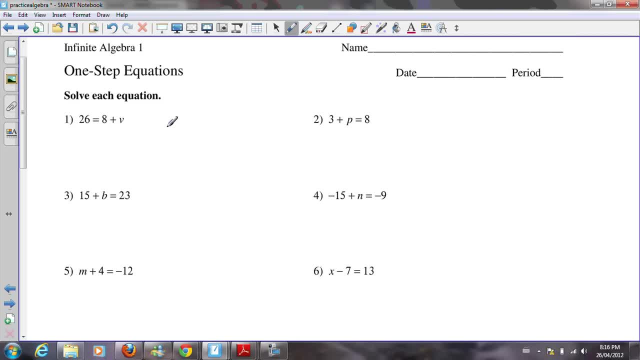 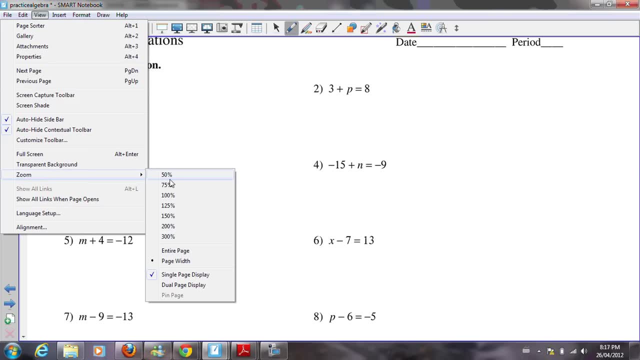 included here. It's called Infinite Algebra 1.. And what we're going to try to do this is starting off with a very simple equation, So I'm going to zoom in a little bit just to make it a a little bit easier to see. oops, this particular problem. Let me see view zoom, let's go. 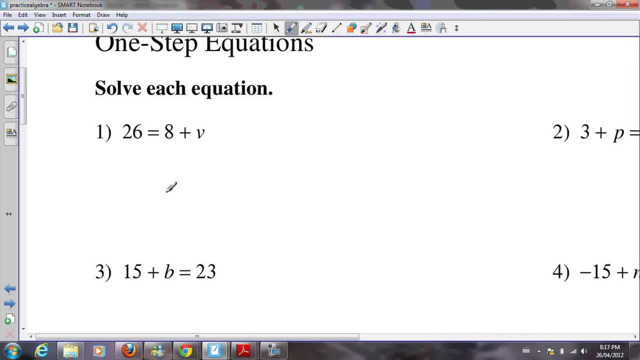 300%, so it's a little easier There. So here's what we have. We have 26 equals 8 plus v, and in this case they didn't use x, they used the letter v. Now we know we want to have. 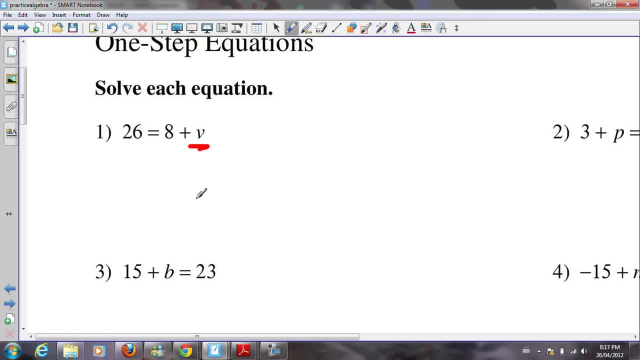 v all by himself in the end. So what is it we want to move? Well, this 8 is going to have to move to the other side. So when we move him over to the other side, a funny thing happens with the 8.. Since we 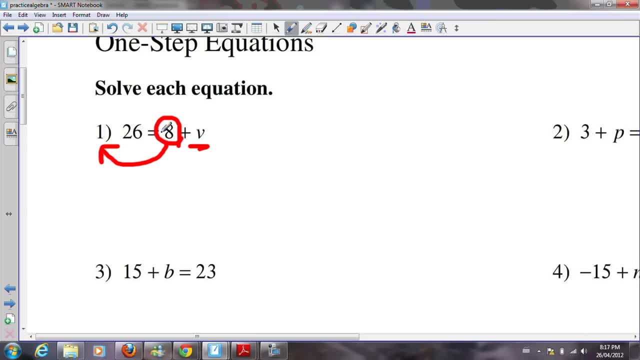 know it's a positive 8, because there's nothing in front of it, there's no minus in front of it. when we move this positive 8 to the other side, we're going to still have 26,, but we're going to end up with this positive 8 becoming takeaway 8.. And don't forget, we 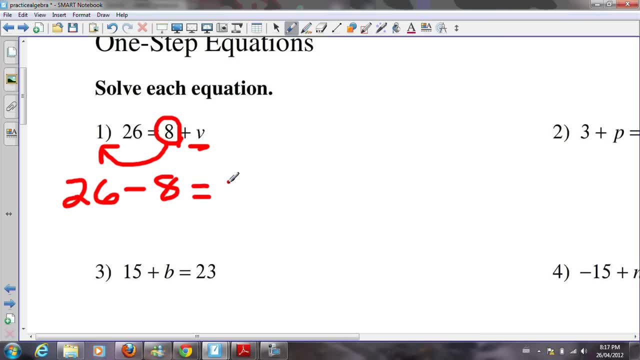 still have this positive v left on this side and I'm just going to leave it as v. Now, when we move 26, takeaway 8, the final answer will be 18 for v. So that will be our final answer. So in ones like this, there's only one step to do. All you have to do is move this guy. 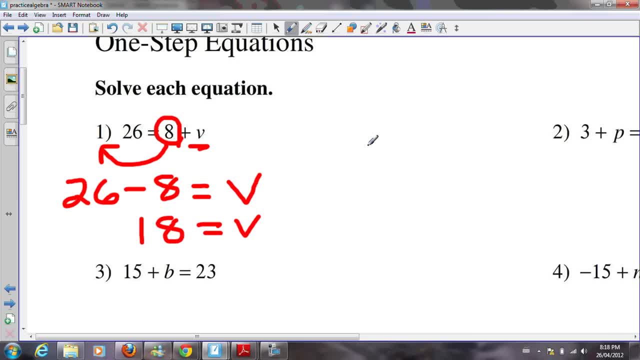 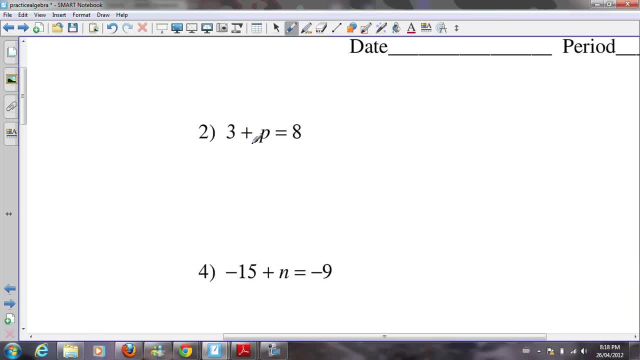 over to the other side and change the sign from a positive to a negative. Looking at a one like this, where the p or the letter is on this side- of course we're not going to move the p over here, We're going to move the number. So this positive 3 goes over to this side and becomes negative. 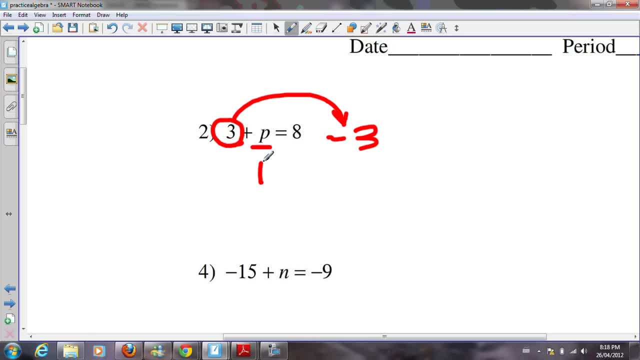 3.. So all we're left with now is p on one side and, of course, 8 take away the 3 on the other. So the answer to p will be 8 take away 3, which is 5.. Now we can easily test out to see if we're right by simply putting 5 back into the original. 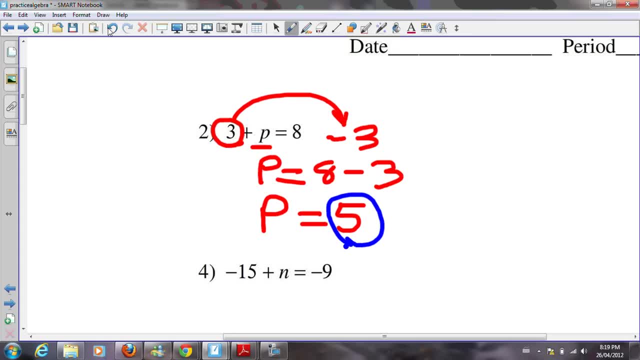 equation for p. So if I go back here and I look at the original equation, which was 3 plus p, equals 8.. So remember our answer was 5.. So 3 plus. let's put 5 in for p and. 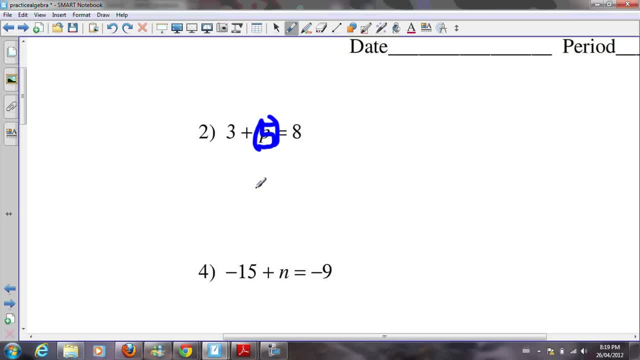 we can put it in brackets, if you want. So 3 plus 5 does equal 8.. So we have 8 on each side. so we know our answer is correct. Now we can put the p in as well, which is 4 and 8.. So we've got our answer here. 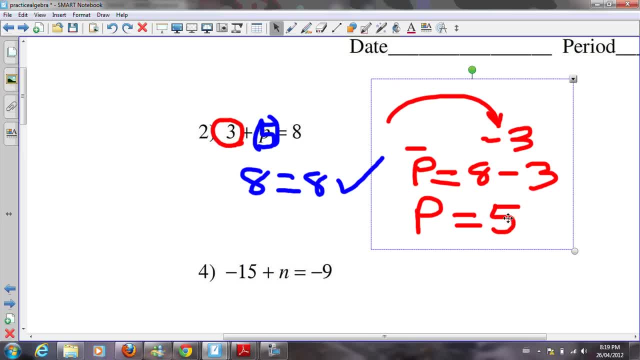 And we can put it in brackets. So here's our answer. So we've got our answer. And let's say we want to get a negative here and we want to get a negative. We want to get a negative, So we get a negative. 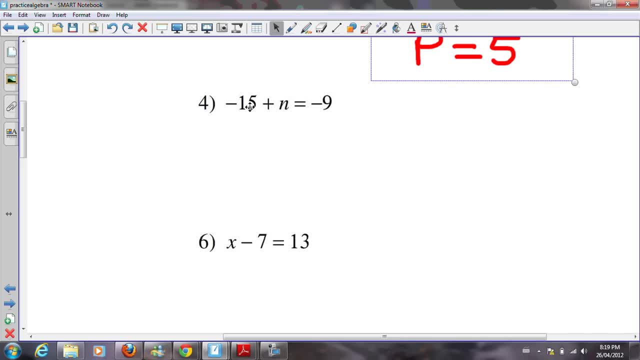 And we want to get a negative. So we're going to need to figure out- and of course, let me move this guy over- That's, if you're asked to validate or check your answer. All you've got to do is take your answer- in this case it's 5- and plug it into your 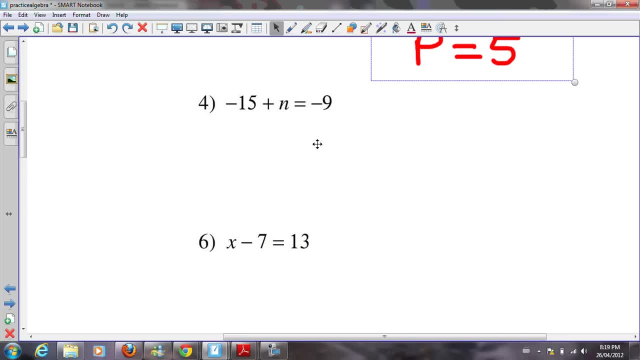 letter. Be careful when you get to negatives here. Sometimes when you put a number to the other side, the negative becomes positive of course. So in this case the minus 15, when we move it to the other side to separate it from the 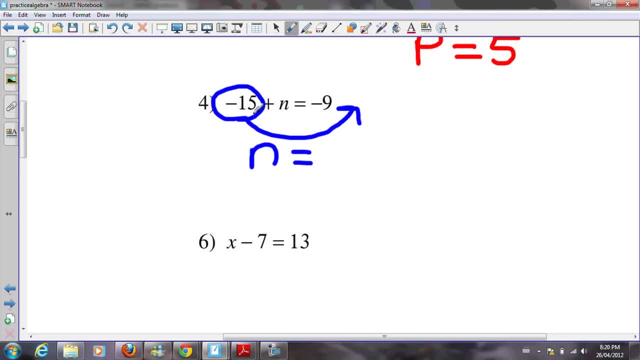 positive n. we're left with n on one side And this minus 15, don't forget, the minus 9 is still there. this minus 15 becomes positive 15.. Now the easiest way to think of when you're doing addition of negative numbers and a positive. 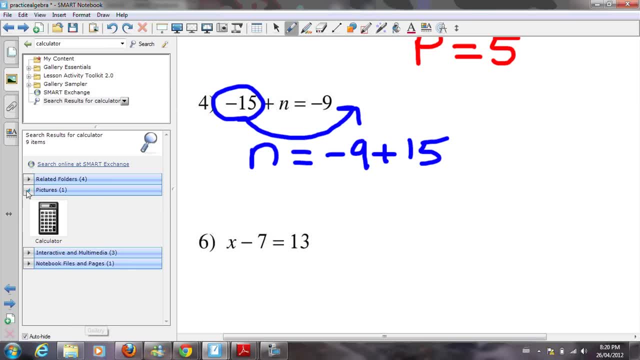 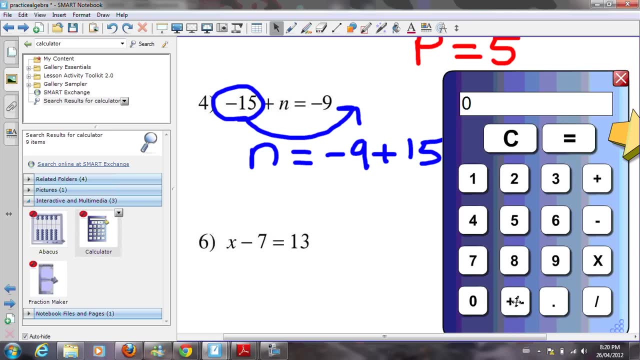 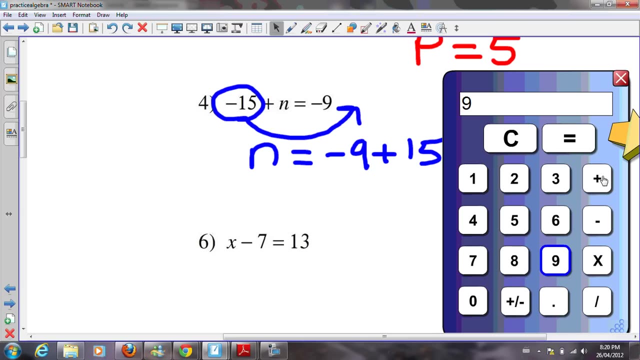 number. you can take out your calculator. in this case, and on most calculators, you will find a positive and negative sign there. So if I want a negative 9,, all I have to do is punch in 9, and then press the positive. 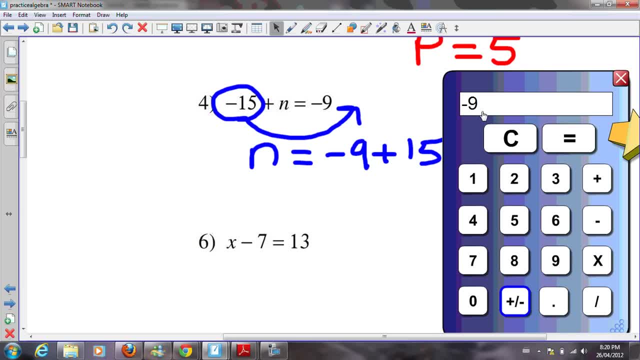 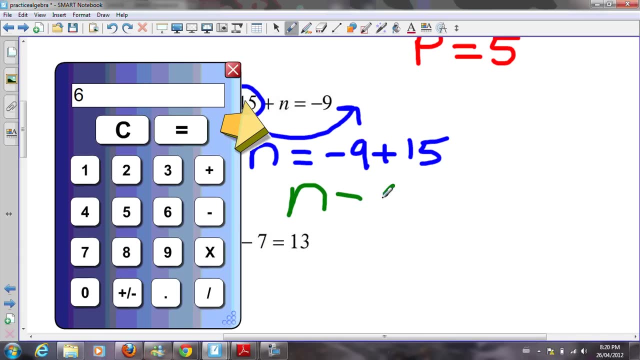 negative 1, and that automatically changes it to negative 9.. And then to add 15,, just go plus 15.. And our answer, of course, for this one, This one, would be 6.. So in this case, n will equal 6.. 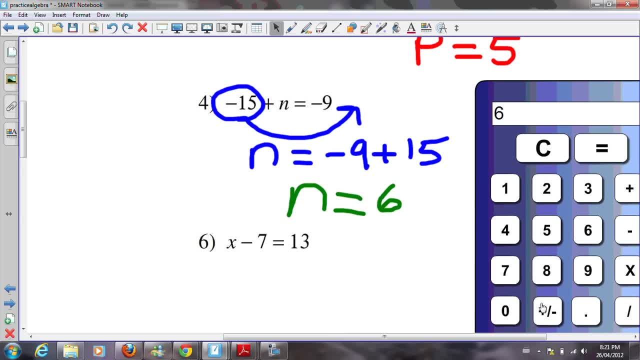 So that's, if you have a calculator that has the plus and minus on it, If you don't just think about it this way- If you have negative 9 on the thermometer- and I could draw a lovely thermometer- and if we're all the way up to negative 9, of course we go up a degree. it's negative 8.. 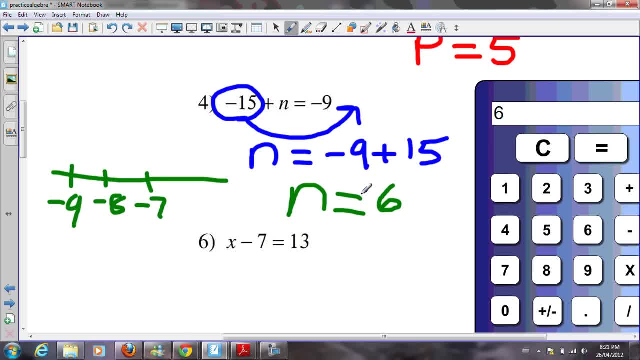 If we go up another degree, it's negative 9.. If we go up another degree, it's negative 7.. So if we go up 15 degrees, we're going to have to jump 1,, 2,, 3, 15 times. 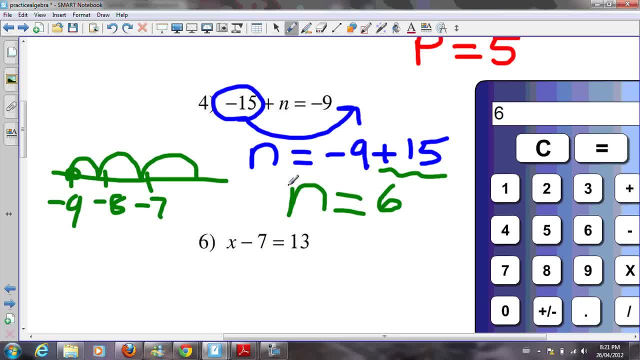 We're going to have to do that 15 times. So you could draw a number line and think of it like a thermometer, And if you're adding you go this way, If you're taking away, you go the other way. And of course, adding a negative, if you have one, is the same thing as taking away. 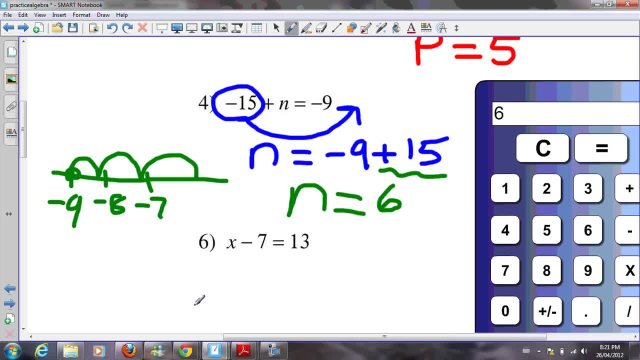 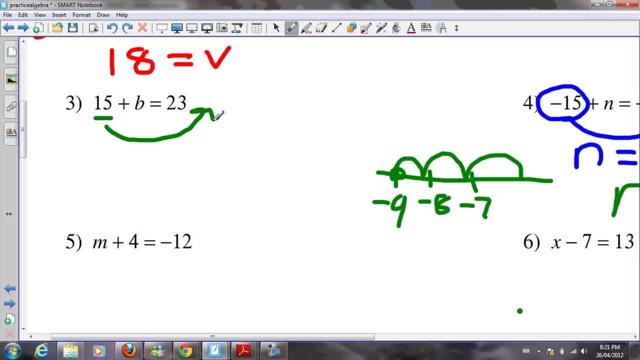 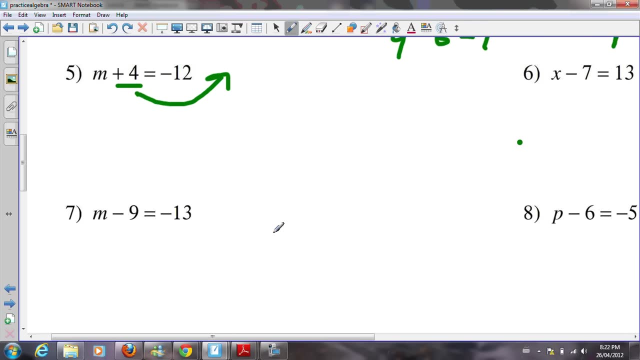 So you can draw: a number line is taken away. So in this case the 15 moves over here and becomes negative. 15. The plus 4 here moves over and becomes negative. 4. The negative 9 moves over and becomes positive. 9. The negative: 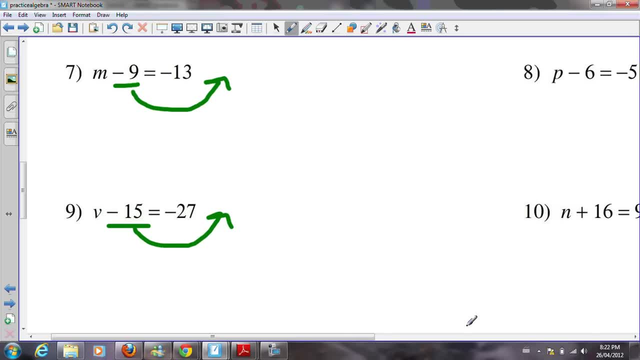 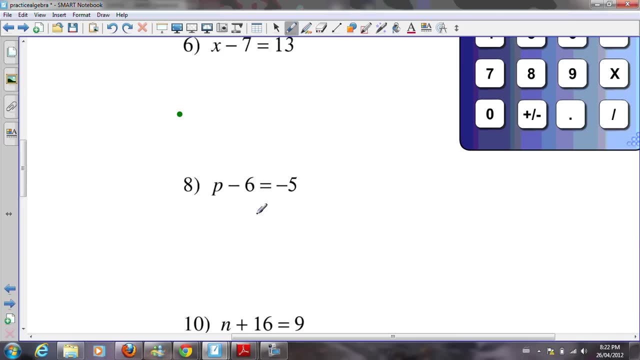 15 moves over and becomes positive 15, and so on. So in just about every one, whenever you have it, whenever you have it and you're trying to figure it out, all you have to do is move the one that's not attached to P. There's nothing attached to P, Just move it over to the other side and change the. 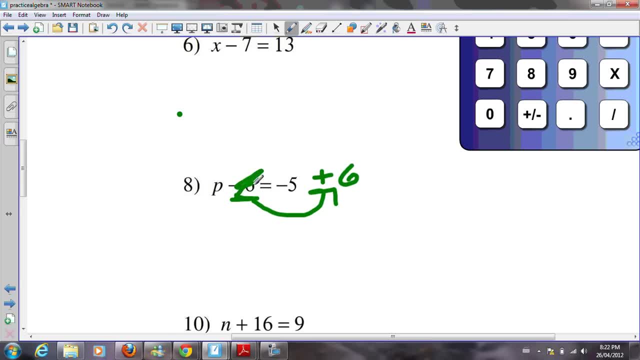 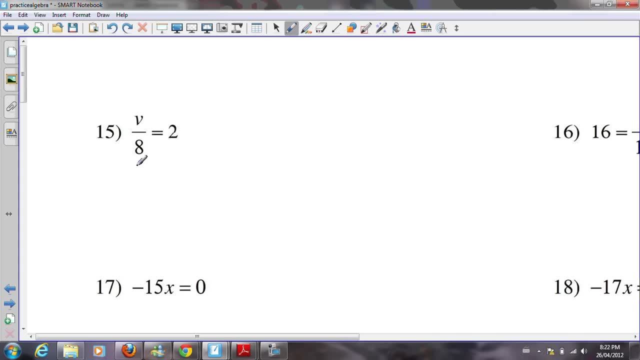 sign to a positive and you'll get your answer. Here's another one. It's a single step one, but it's not plus or minus. You'll notice that it's a fraction. So in any fractions written like that, what this fraction really means is divided by. 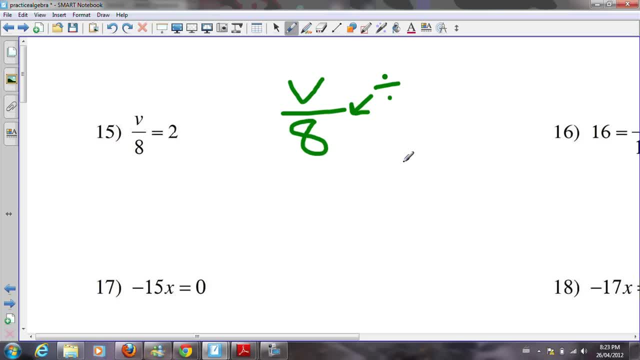 and to find what the opposite of divided by is, you just have to think of multiply. So if you have V over eight and you're dividing by eight And you've got to times it by 8, or do the opposite, That will cancel it out for you. 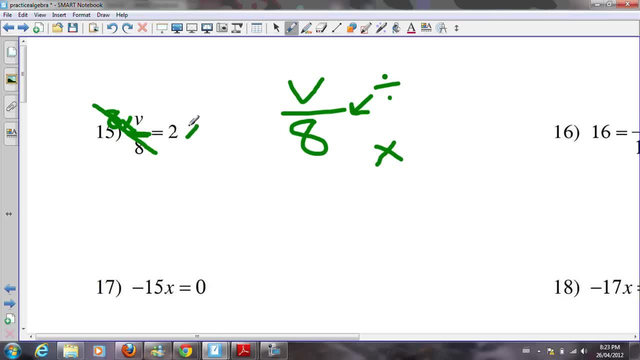 But don't forget, whenever you do it to one side, you must do it to the other side. So we have v left all by himself, And 2 times 8, which is 16.. So we just solved for v. v will equal 16.. 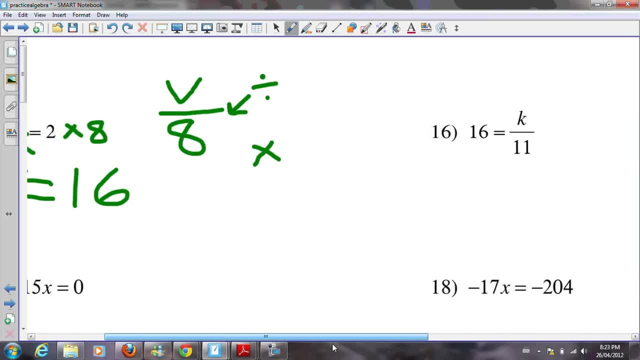 So I could show you that one in another one here. There we go. So we got 16 equals k over 11.. I think I'll put that one on another page. So 16 equals k over 11.. So we want to get rid of everything on this side. 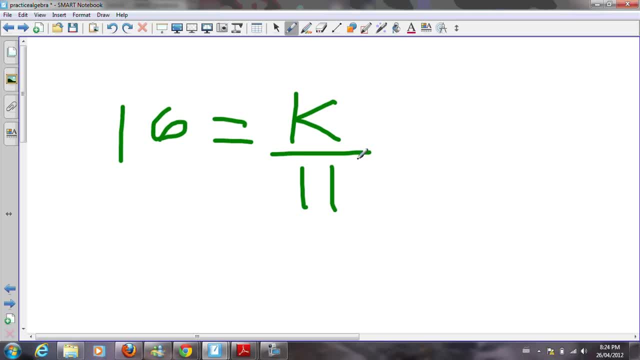 except for the k. Well, since this means divided by a fraction is divided by, we're going to do the opposite And we're going to multiply by 11.. That will cancel out, of course, the 11s, Because 11 over 11 is going to equal 1.. 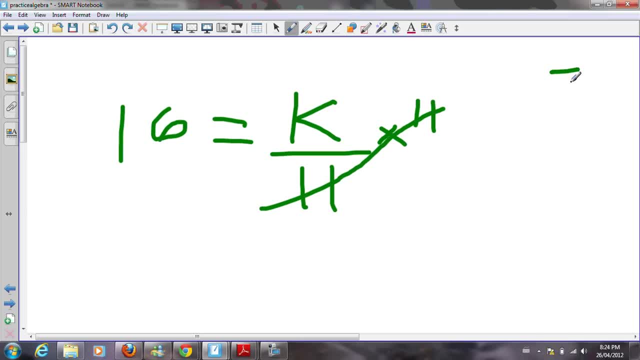 Any time you have a fraction, that is say even 7 over 7,, that equals 1.. 20 over 20 equals 1.. So don't forget, though, When you times one side by 11,, you must do the exact same thing to the other side. 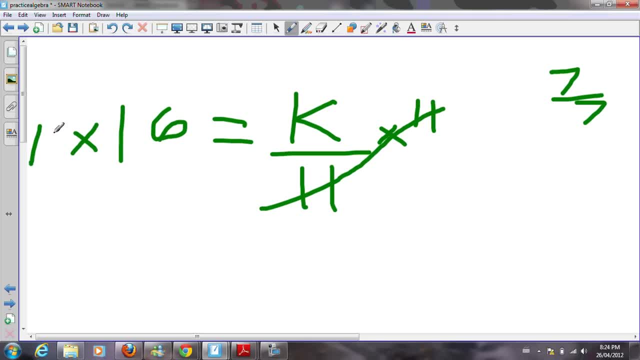 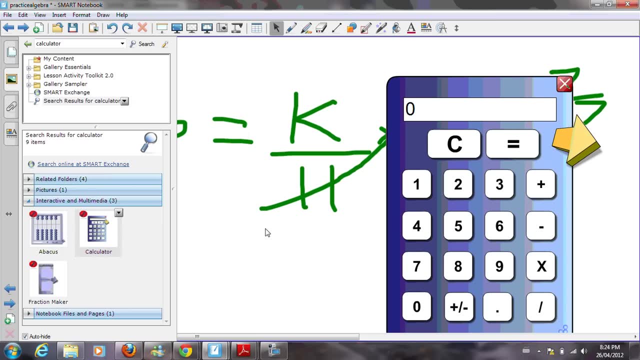 So I'm going to have the times 16.. So I'm going to have the times 16 by 11 as well. So I'm going to take my calculator, move him over here And of course, then I'm going to go 11 times 16.. 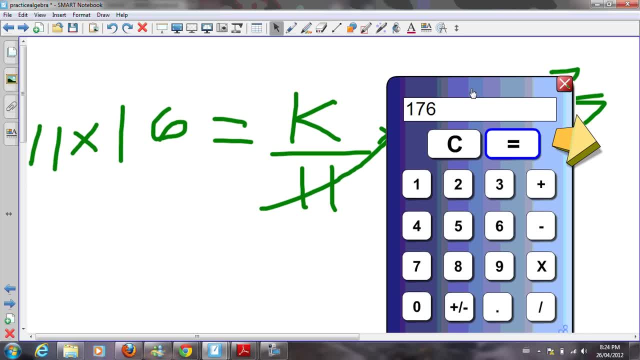 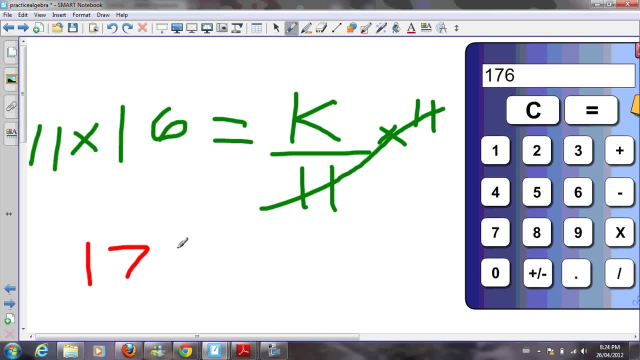 And my answer, of course, is 176.. So my answer to this math problem, just by using the calculator, will be 176 left on one side And the other side is just k, So k equals 176.. It doesn't matter which side you put the k on. 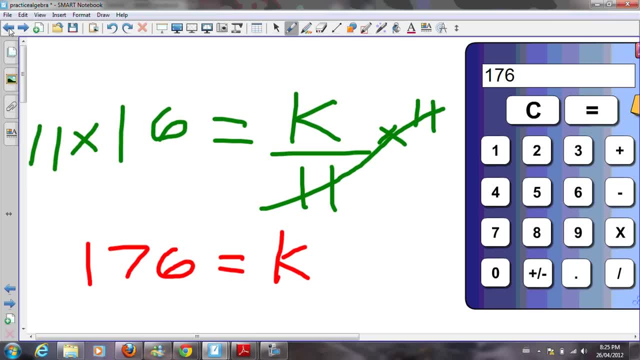 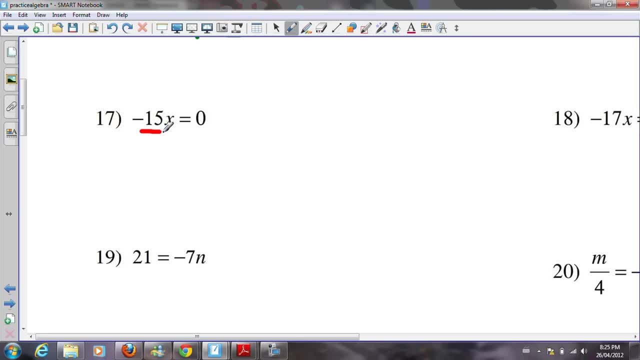 or which side you put the other one on. Sometimes you'll see it written both ways. Looking at this one, this is not a divided by. There's no divided by. underneath that, There's no fraction. So whenever you see just the numbers touching the letter, 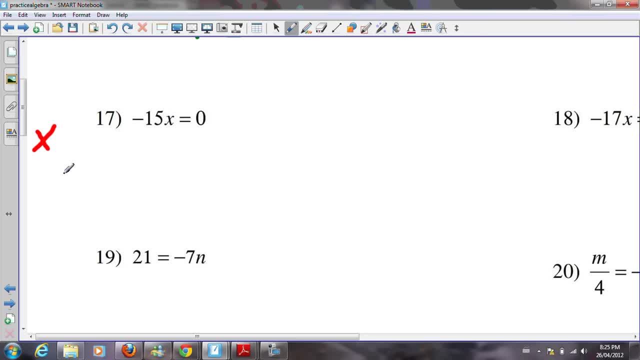 that really means multiply And of course we're going to do the opposite. So when you've got negative 15 times, we're going to go and divide it by negative 15, like that. That will cancel out the negative 15.. 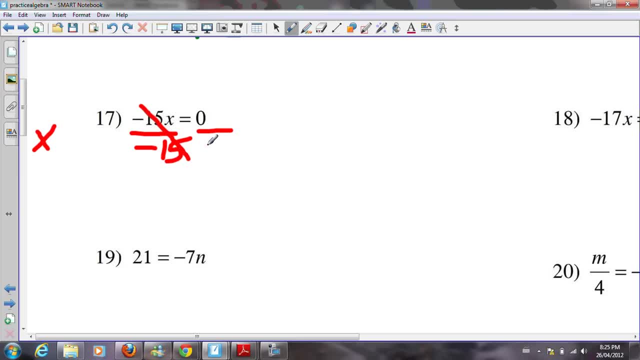 Don't forget: what you do to one side you must do to the other. So I'm going to divide 0 by negative 15.. And it doesn't really matter When we solve that: 0 divided by anything is still going to be 0. 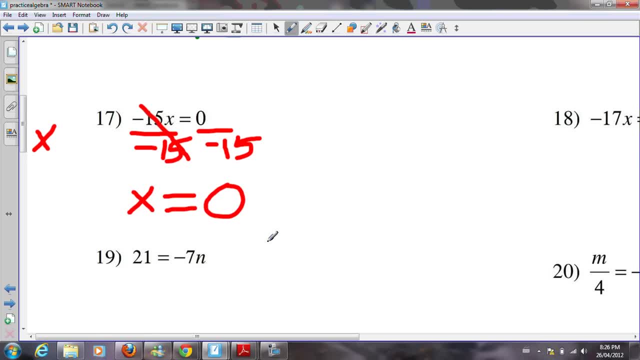 So x will equal 0 in this case. Let's keep going, Let's keep going. Looking at number 19, there's a negative 7 in front of n, So you've got to divide it, because negative 7 is times n. 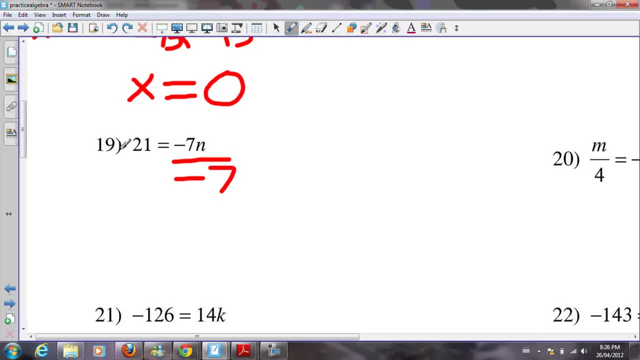 So you must divide it by negative 7,, like that. And of course you do it to one side, You cancel out the minus 7.. You must do the exact same thing to the other side, So we're left with just n on one side. 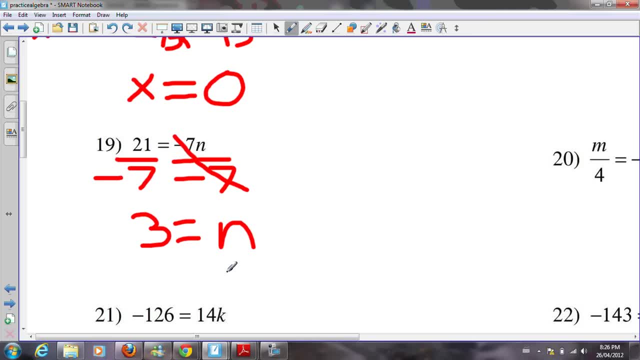 And 21 divided by 7 is 3.. And you can use your calculator for that, But don't forget, it's a positive 21 divided by a negative, 7.. So a positive divided by a negative is always a negative. The only way you can get a positive out of a negative. 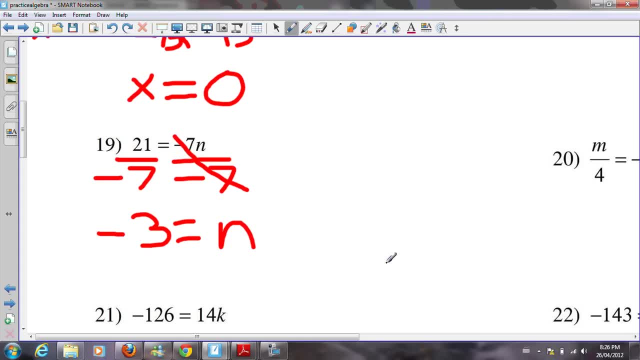 is if both of them were negative, which they're not, So we're not going to put it there. So in this one here, since that's 14 times k, we're going to divide it by 14 on each side. Moving over here. this is negative 11x. 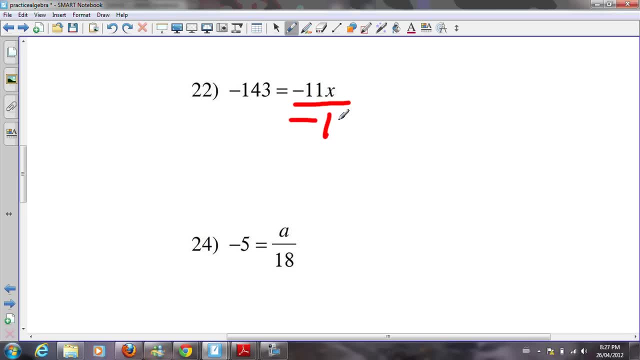 So we're going to divide it by negative 11 in order to cancel it out, And then we're going to divide this by negative 11 on this side. So a negative divided by a negative is a positive. So we know our answer's going to be positive. 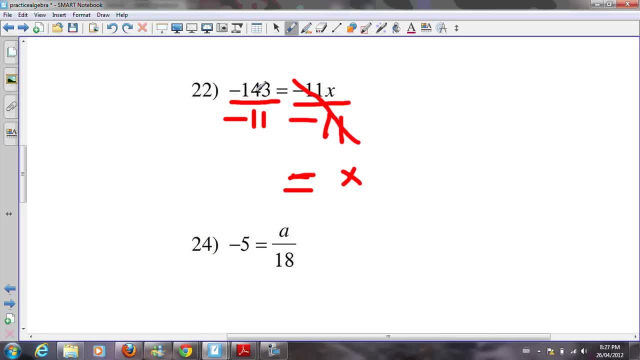 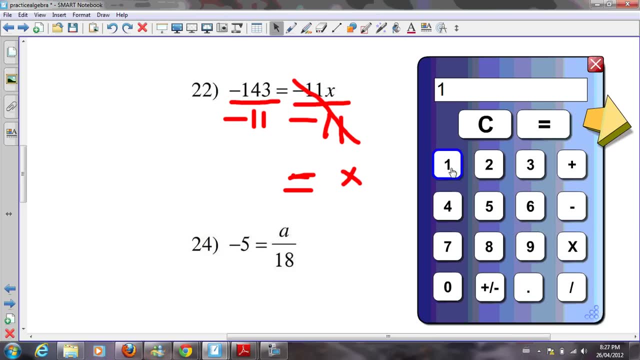 So x is all by himself now 143 divided by 11, if I were to take my calculator, So 143 divided by 11.. And you notice I didn't put in the negatives when I did it, because I know a negative divided by a negative is a positive. 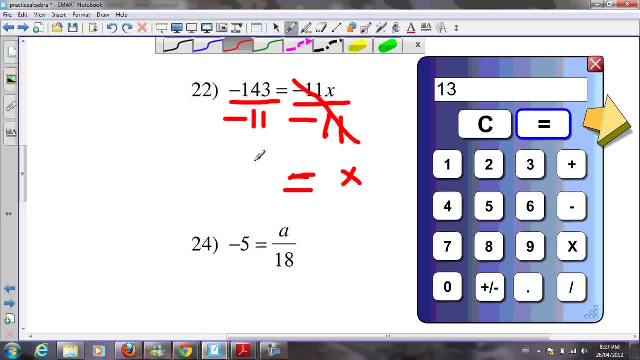 So I don't need to worry about my negatives, But my answer does turn out to be 13.. So if we put x back in there, if we put 13 times negative 11, we should get negative 143.. So we could always check. 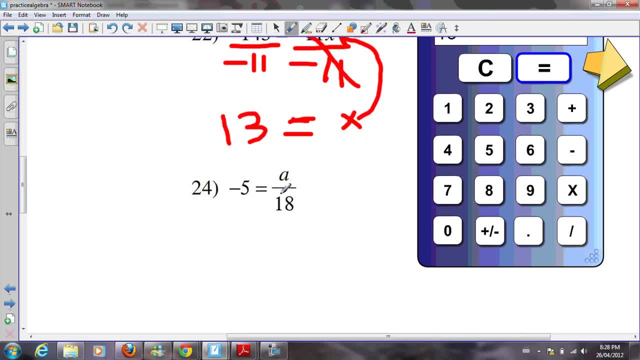 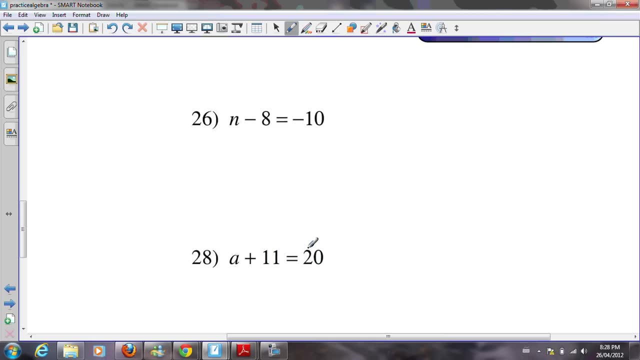 Let's check our answer. So this one here is divided by 18.. So we're going to times it by 18 to cancel out this side. Of course, you must times this minus 5 by 18 to cancel out, or sorry, to get your answer on that side. 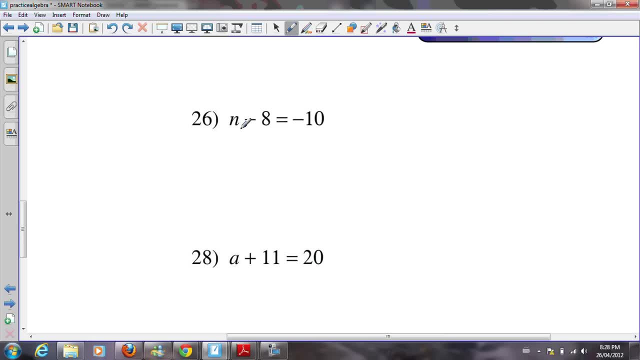 So it's pretty much the same thing all the time. You're either going to have to shift If it's a take away or plus, you're going to have to shift it over to this side and change the sign If it's a divided by. 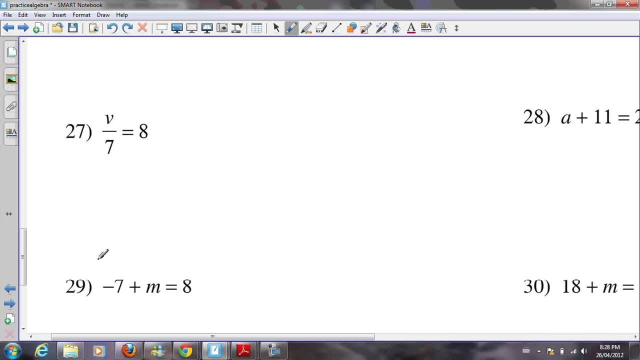 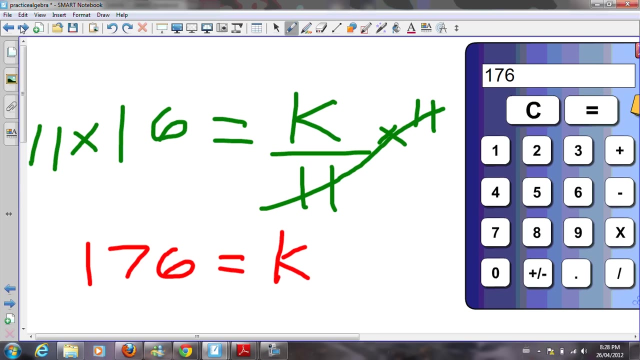 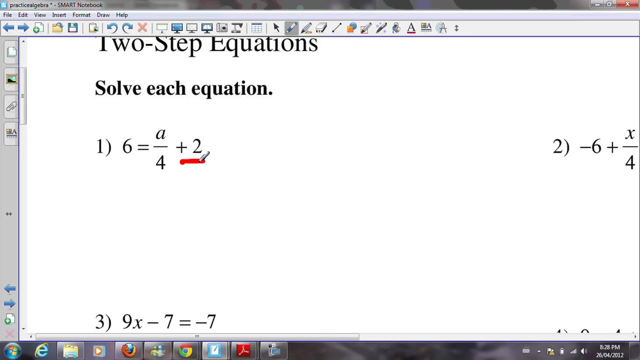 or a multiply. you're going to have to do the opposite and times it by 7, or times it by a number, Or, in some cases, you'll have to divide it by a number, like we did up here. All right, so now that we know how to do the shifting of numbers. 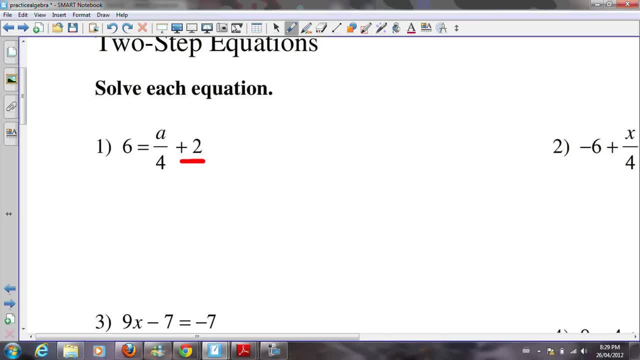 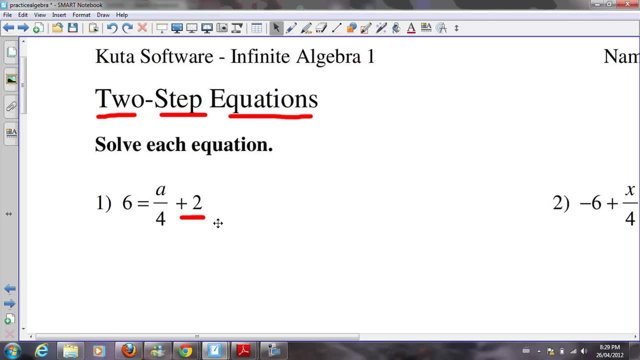 and we also know how to multiply the numbers. sometimes you might get two step equations, And these are usually the ones that are worth the most on a test. In these two steps you just got to do one step at a time. It's no big deal, no harder. 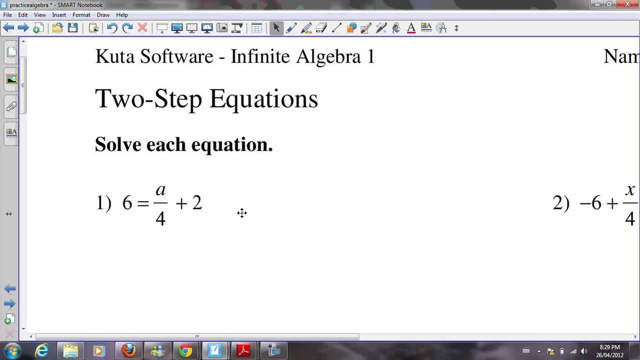 It's just you got to remember which step to do first. And in this case we always move what's not connected to the letter. So this a over 4, we can't just take the a off and move them over here because he's part of a fraction. 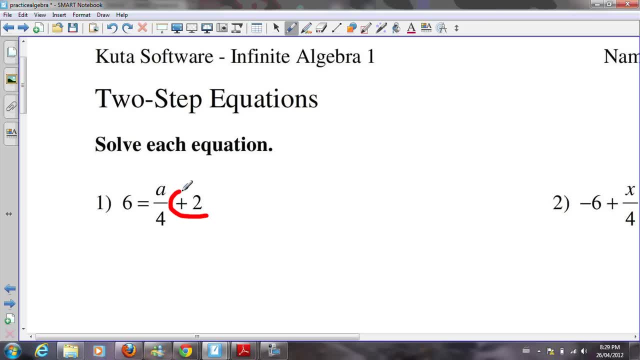 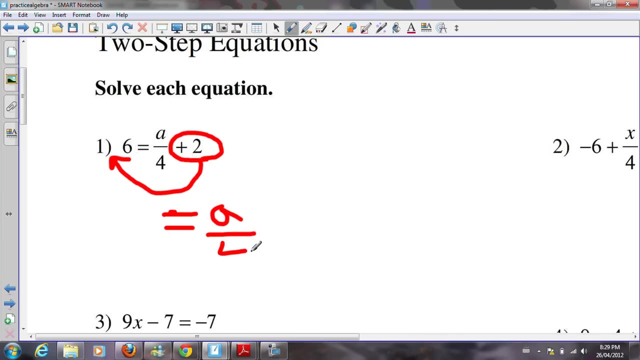 So we're going to keep him there and we always move the plus or the minus first, So I'm going to take this plus 2 and shift him over to this side. So I've still got a over 4 left on the right-hand side. 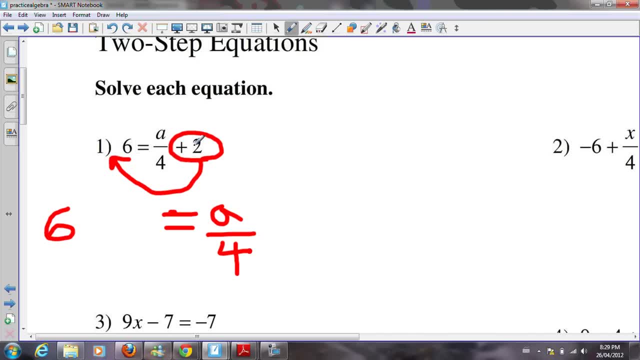 On the other side. since I've moved my positive 2 over here, the sign changes to a negative 2.. So 6 take away 2 is 4, and we've still got that a over 4 left. Now the easiest way to get rid of a divided by 4 that's down here. 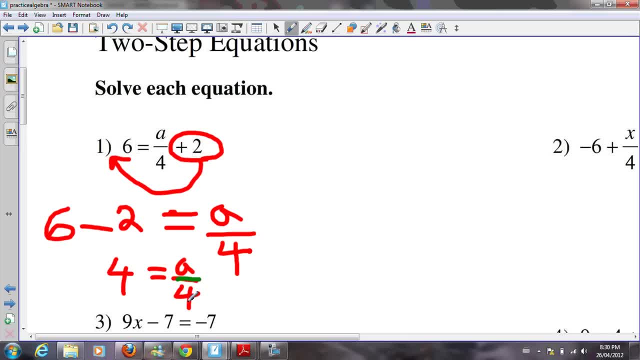 because that's the only thing left: the divided by 4. Is to times it by 4 to cancel it out. And of course, if you times one side by something, you must do the exact same thing to the other side. So a is all by himself on one side. 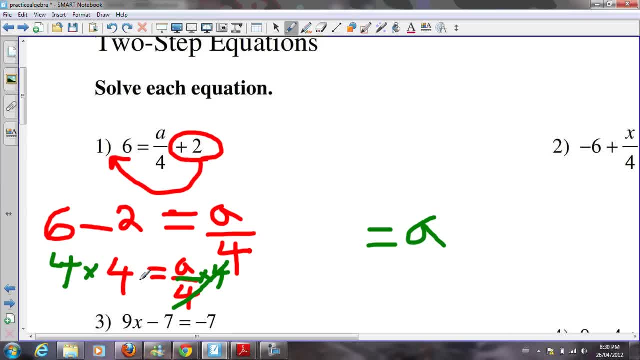 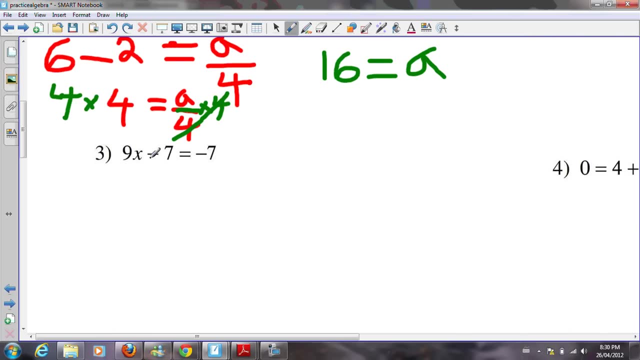 And of course, four times four, one going to 4.. will give you 16 on the other, So a must be 16 for this equation to be true. Looking down here at this one, maybe I'll do him on a separate page again. 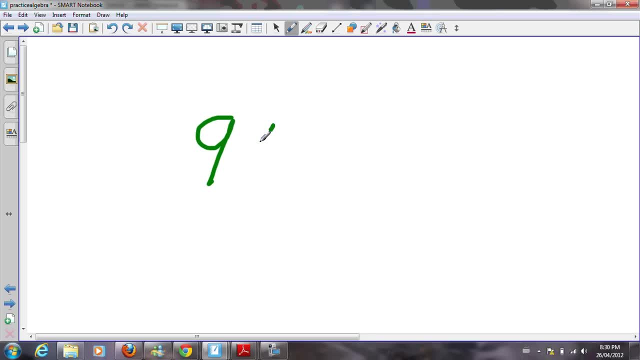 9x, take away 7.. So 9x, take away 7, equals. and just to double check, 9x, take away 7, equals negative 7.. So remember, the first step always is to deal with the thing that's not connected to the x first. 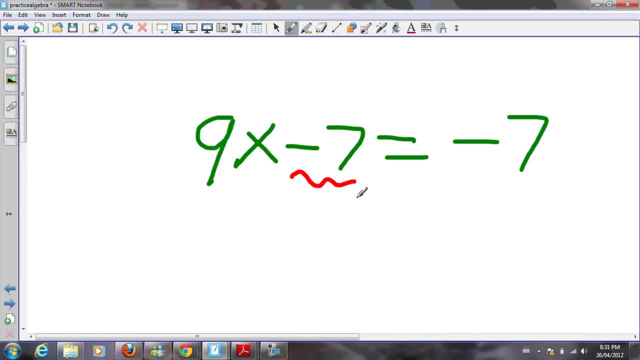 In this case it's the minus, or to take away 7.. So I'm going to shift him over to the other side and he's going to become plus 7, because he switches signs. So we're left with 9x all by himself. 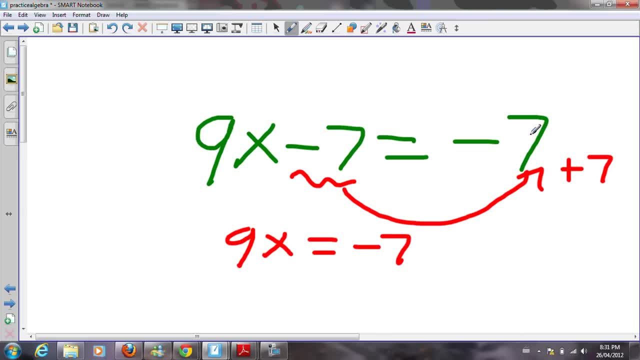 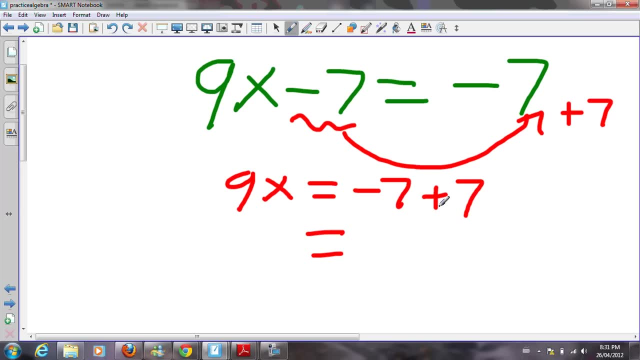 equals negative 7 still there and we've also brought over a plus 7.. All of a sudden, negative 7 plus a 7, they cancel each other out to give you 0. Because if you have a negative 7 degrees, 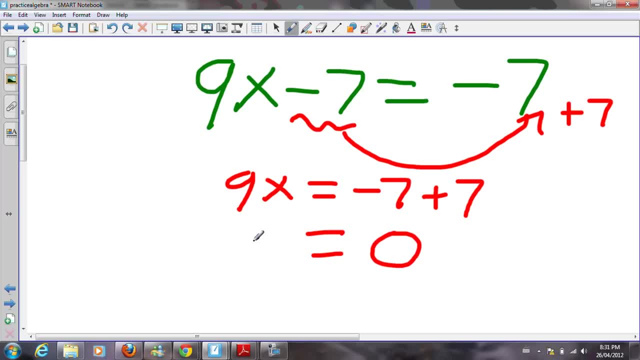 and you add 7 degrees, you're back to 0 degrees And of course 9x is still here. And to get rid of this 9 times x, we must divide it by x And of course we know 0 divided by anything. 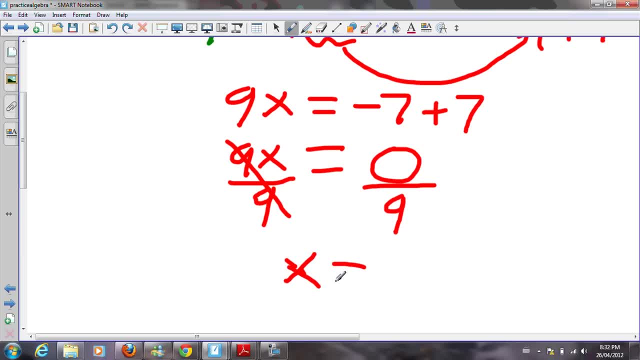 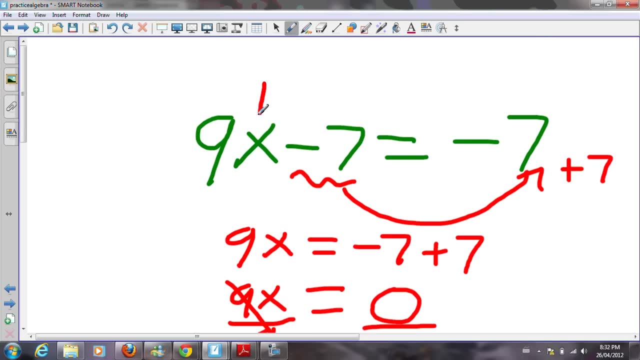 is still going to be 0. So x will be 0 in this case, and that makes sense, because if you put 0 back into x up here, 0 times 9 is still 0, so that cancels it out. 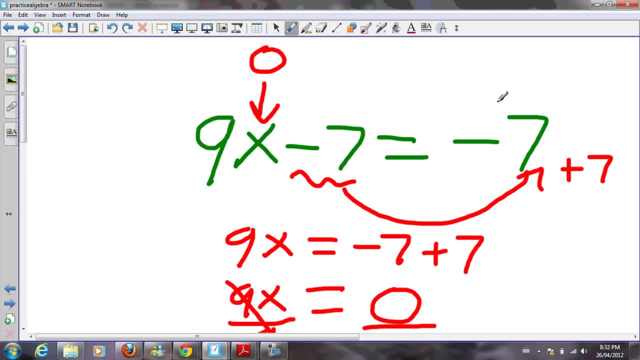 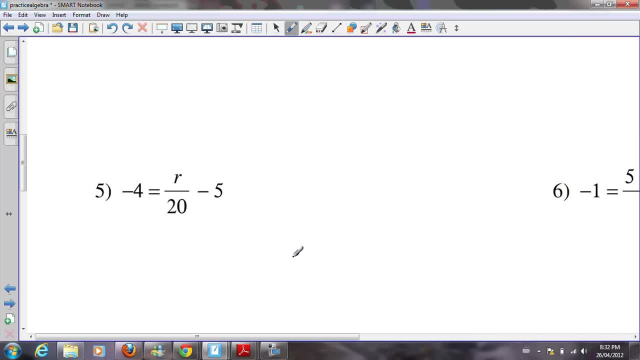 And we're left with just negative 7 on this side, which is what we've got on the other side. Okay, in this one here it looks a little harder, but it's not really. The first thing we deal with is the. 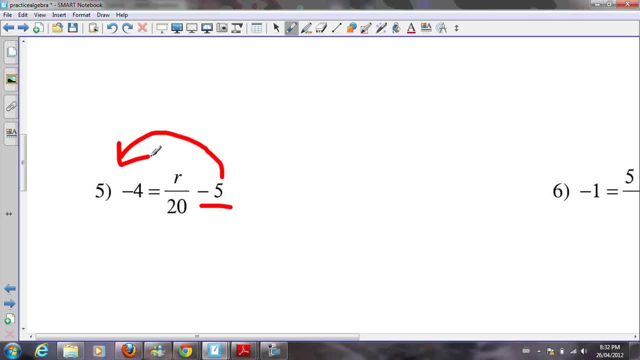 plus or minus. So we'll take the minus 5 and bring him over here. So negative 5 now becomes a positive 5, because we shifted them. So negative 4 is still there, plus 5 equals- and remember, this is still on that side. 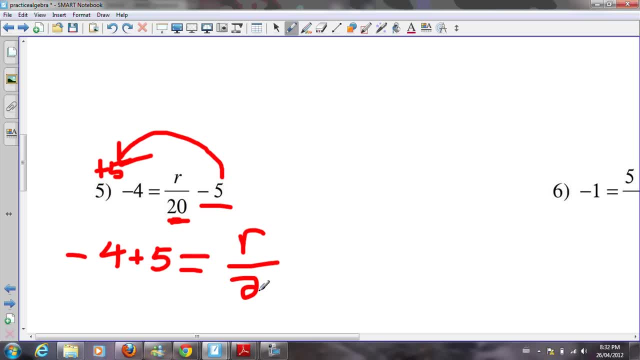 r over 20.. So negative 4 plus 5,, if you punch that into your calculator- is positive 1. And that equals r over 20.. The only way to get rid of that divided by 20 now is to do the opposite. 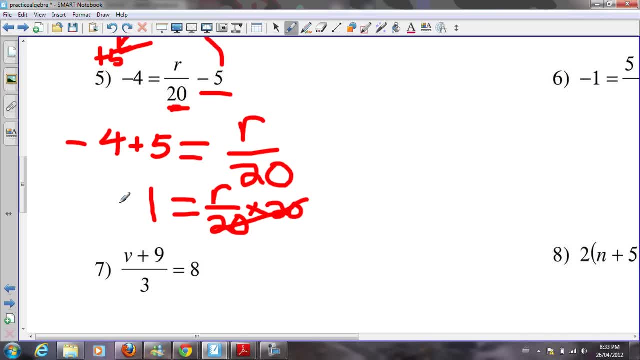 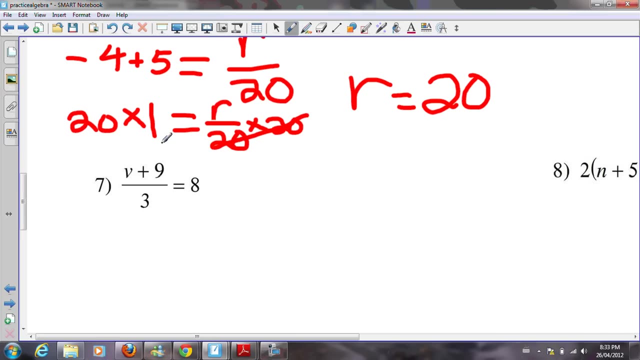 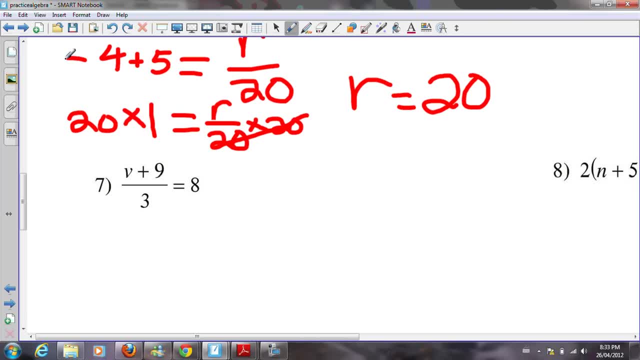 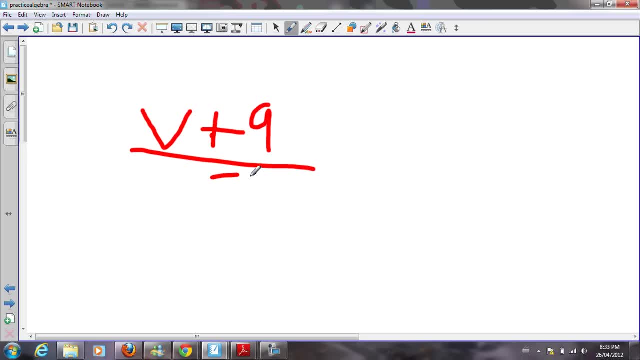 Okay, Okay, Okay, Okay, Okay. So 1 plus 9 over 3 equals 8.. So that one's a little bit trickier. So V plus 9 over 3 equals 8.. Just to double check. 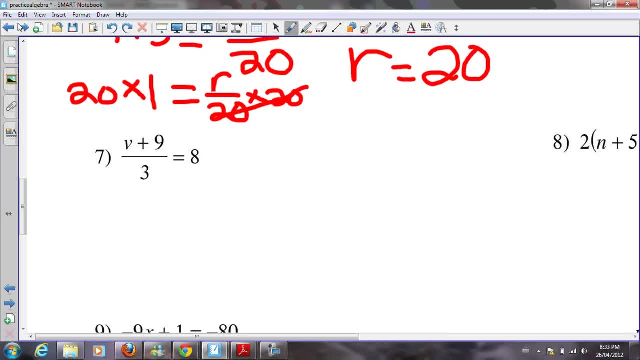 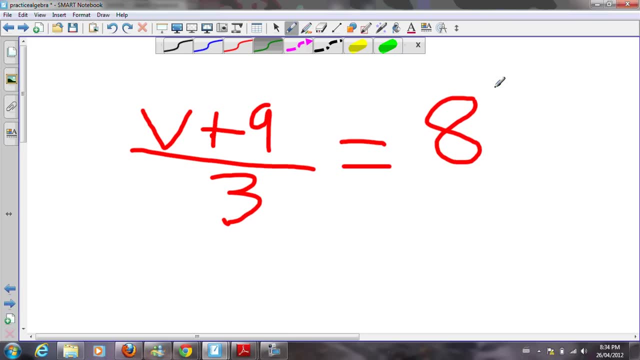 make sure I wrote that down correctly: V plus 9 over 3 equals 8.. So again, you would almost think you've got to move this plus 9, 9 over here. but the problem is this: V plus 9 is part of this whole fraction. 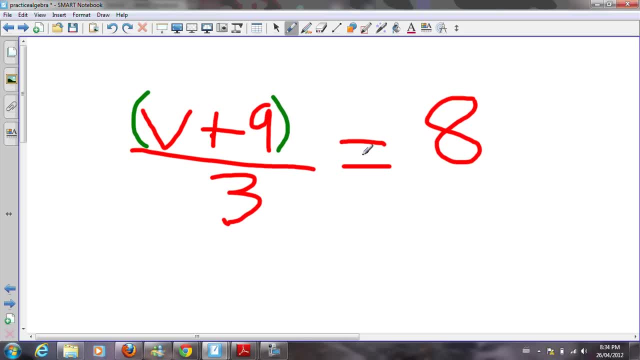 okay, so it's like having it in brackets. so how do we get rid of the divided by 3? first of all, and the easiest way to get rid of the divided by 3 is to times each side by 3. of course, that will cancel out the 3 and we'll times this by 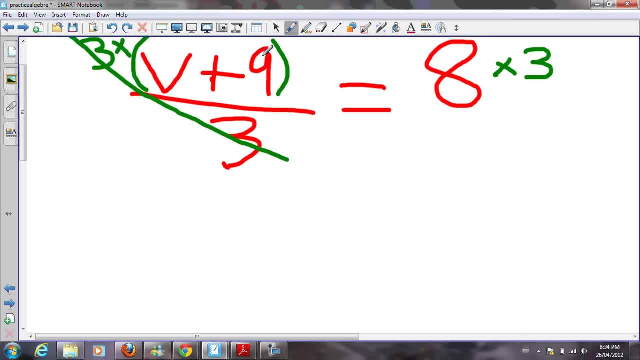 3 on this side. now we're left with V plus 9 on one side, 8 times 3. if you work it out on your calculator will give you 24. now it looks like one of those one-step problems that we were doing earlier. so we take the plus 9, bring them. 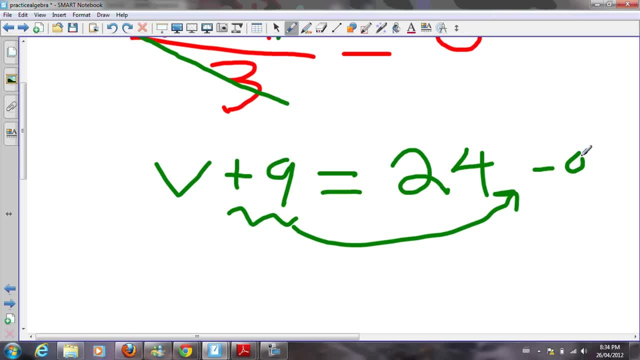 over to the other side and shift them and it becomes negative 9. so V is all by himself 24. take away 9 will leave us. well, you take away 10 and it'll be 14. so add one more and it'll be 15 for our answer. so remember: anything in brackets needs to. 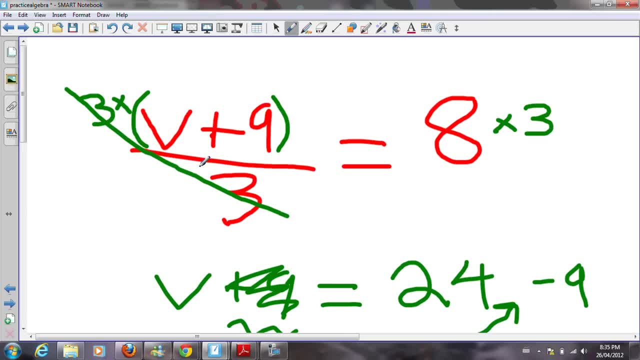 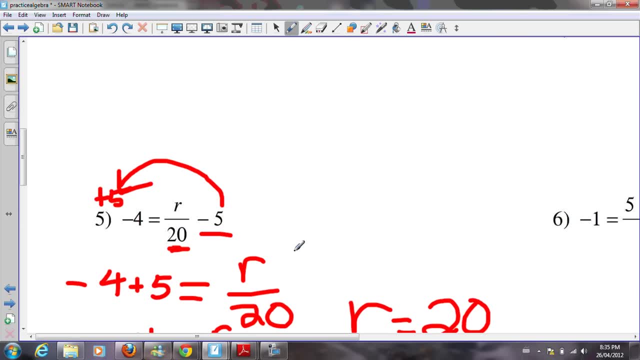 stay together, you still times it by whatever you need to times it by to get rid of the divided on the bottom. okay, so let's try another one, and I think I'll try this one that I'll get rid of This one that already has a 1 here, so this one here is 2, and then bracket n plus 5. now 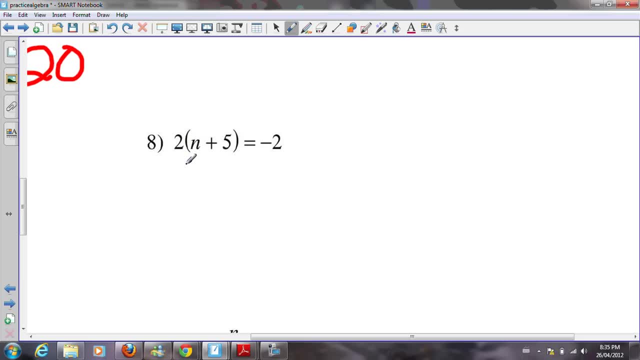 you could go ahead and work it all out, but there's no, really no need. all you need to think about is how do I get rid of this 2 times all this stuff on that side? and the easiest way is to just divide it by 2 and that'll cancel out that. but if you do it to, 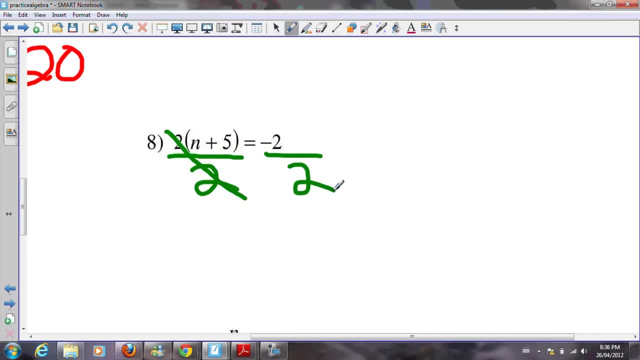 this side of the equation, you must divide the other side by 2.. So we're left with n plus 5 equals well, 2 divided by 2 is 1 and a negative divided by positive is a negative. so now all we have to do is shift this plus 5 over to the other. 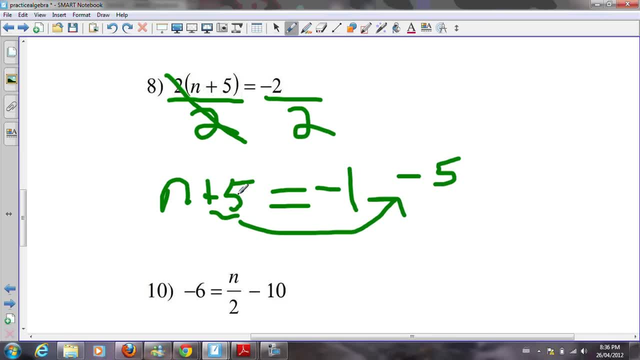 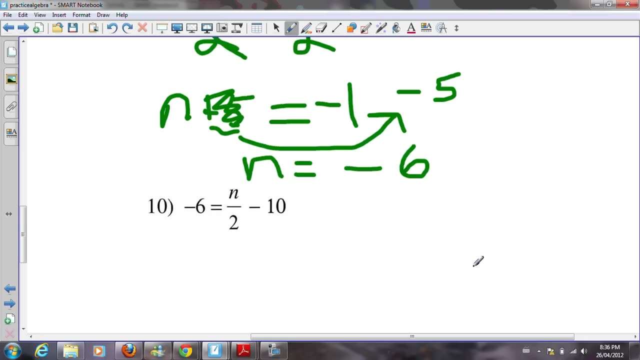 side and it becomes negative 5. that gets rid of it. now we're left with n equals negative 1.. So we're left with n plus 5 equals negative 6, and that will be our answer for that one. So in these two-step problems you always start with the plus or minus first and shift him. 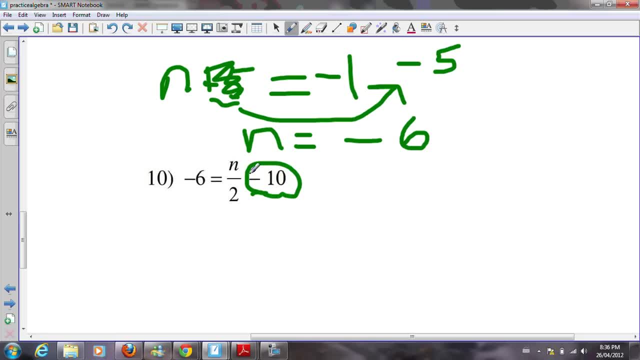 over, and then you've got to times it by a number, or sometimes you got to divide it by a number, depending upon what the opposite is. So, as you can see, all of the problems On the example sheets are pretty much the same. you shift them over and then, of course, 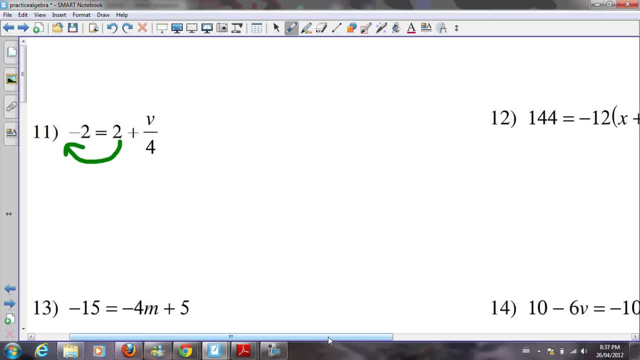 you're going to times it by 4 to cancel out the divided by 4.. If there's brackets, well what's in front of the bracket? this is 12 or negative 12 times all this. so we're going to go divided by negative 12 and that'll cancel that. and of course then 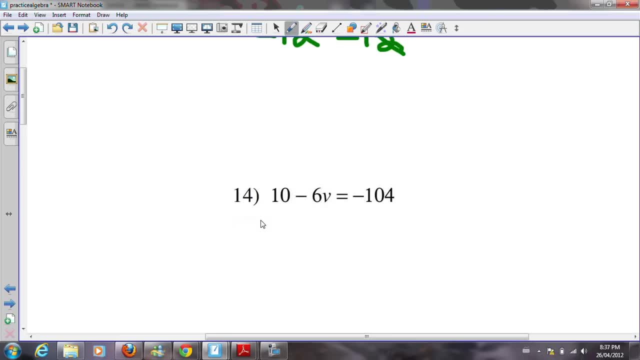 it'll be much simpler to solve. Be careful with your negative signs. You must shift this over first and it becomes positive, and then you've got to divide by negative 9 to get rid of the negative 9 times. So don't forget to do not just the nine times but the negative that's in front of the. 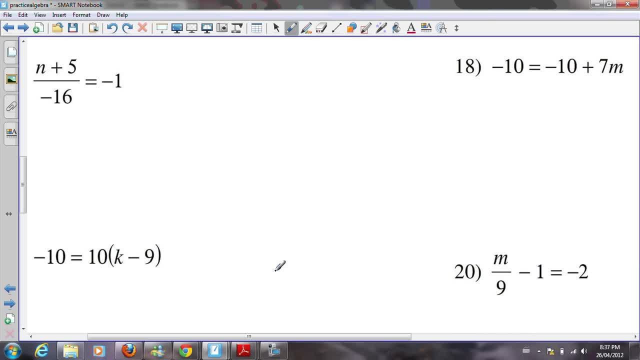 nine as well. Last one over here: Choose the kali recruiting button From all these buttons. Yeah, We're just going to fill them in and create, just for you, di rolls, and then we're going to change everyone to anything from that part over to the other side. 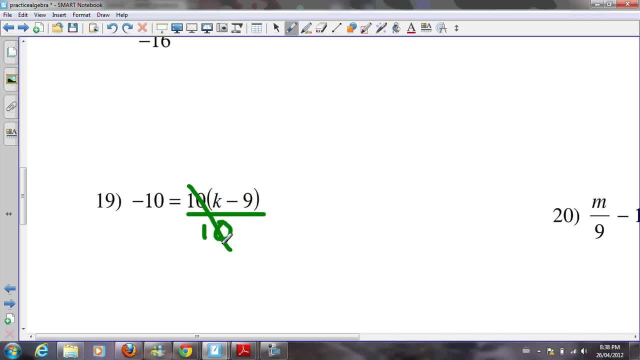 You've got to divide it by 10 to get rid of the 10 in front, but don't forget to do it to both sides and watch your negatives when you're doing this one, and it should work out for you nice and easy. 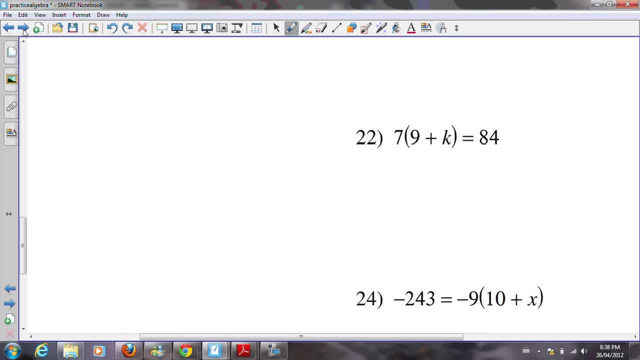 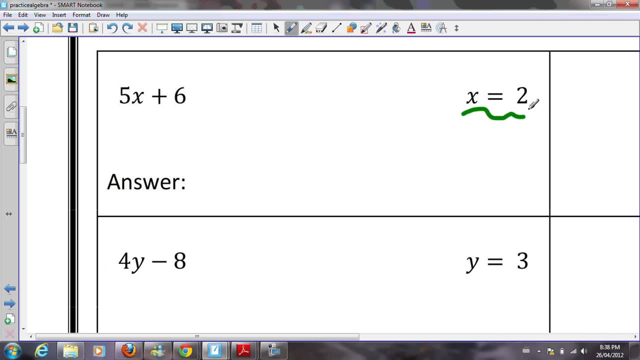 just like the rest of them. You might be given sometimes the value of x and you might be asked to plug it back into your equation. It should be easy. Just take 2, and wherever your letter is, it doesn't have to be x. 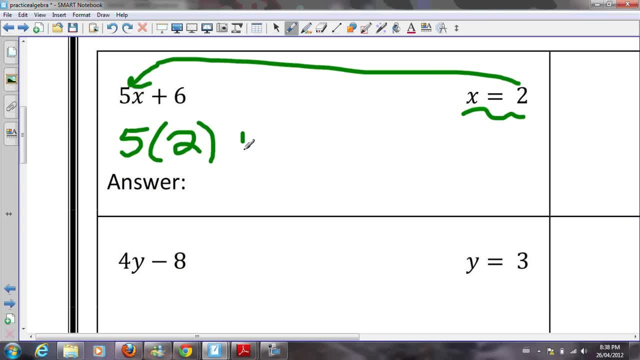 just simply put 2 or whatever you're given into it and solve it like you always do. So 2 times 5 is 10, plus 6 more is 16.. So the answer, when you put x in, there will be 16.. 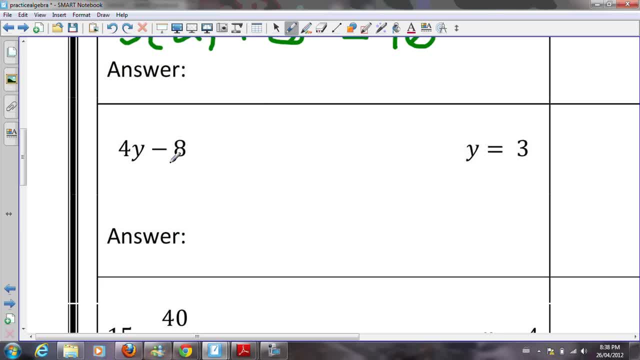 When you're looking at this one here, we could use y. Usually we stick to x's. We stick to x's and y's in math. Put 3 in for y and of course, 4 times 3 is 12.. 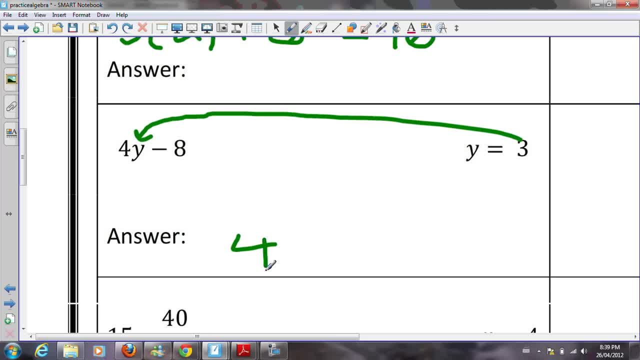 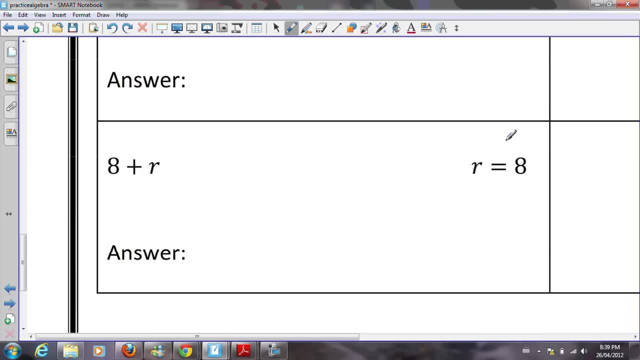 Take away 8, we'll give you 4 for your answer. All the answers are given to you anyway, so this is just a practice that you can go ahead and work on Now. why do you need to know how to plug in certain numbers? 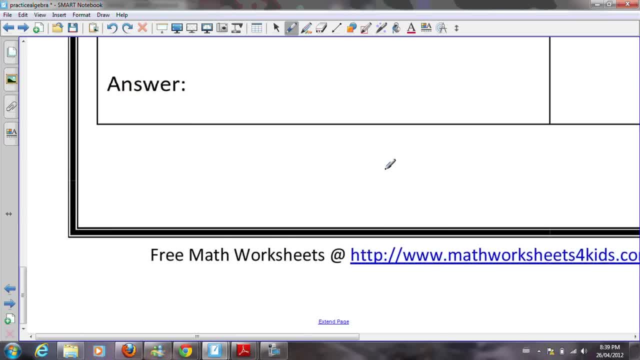 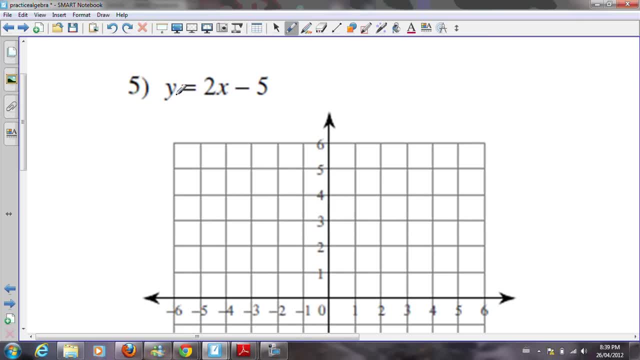 and solve and get an answer, Because when you start the graphing coming up next, you're going to be given something with x and y and you're going to have to plug in your own numbers. So I'm going to zoom back out just a little bit. 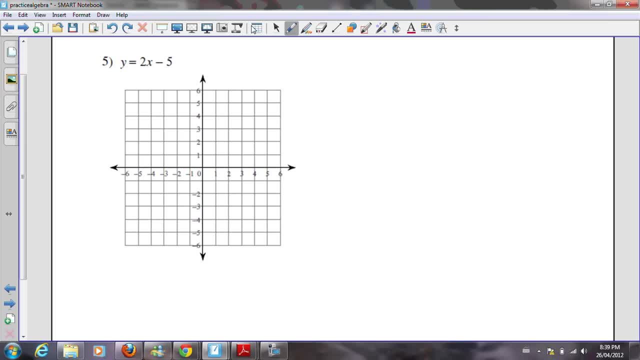 and we'll go out to there, and that should give us enough so we can see it a little bit clearer. So here's what we've got. We've got y and x, so we've got two letters. Now you remember back in grade 5 and 6,. 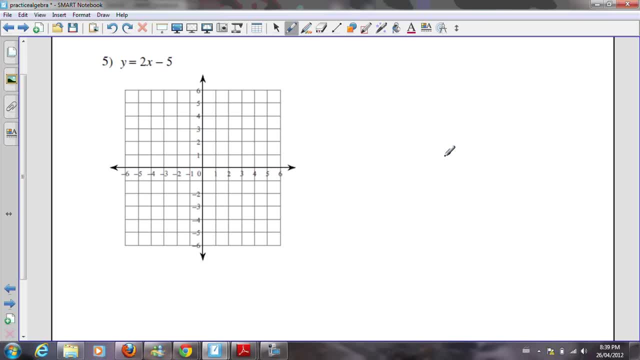 you guys had to do these coordinate planes. It's almost like playing a game of Battleship where you had to call out two numbers, or a letter and a number 52. So you looked at b on one side and you looked at 52 on the top. 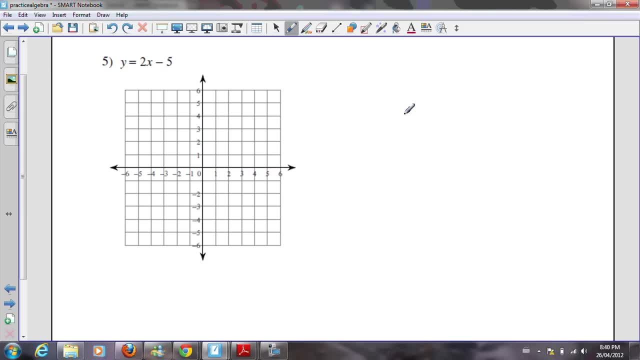 and then you matched them up in order to see if you could sync someone's Battleship. What you're really trying to do here is come up with your own values and then plug it into this chart. Going left or right is called the x value. 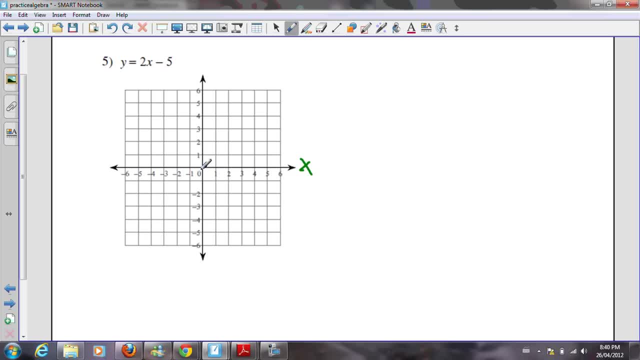 So if it's positive, you go this way, If it's negative, you go that way first. So you always go sideways first. for x, For the y value on this graph it's the line going up and down. So if your answer or y, 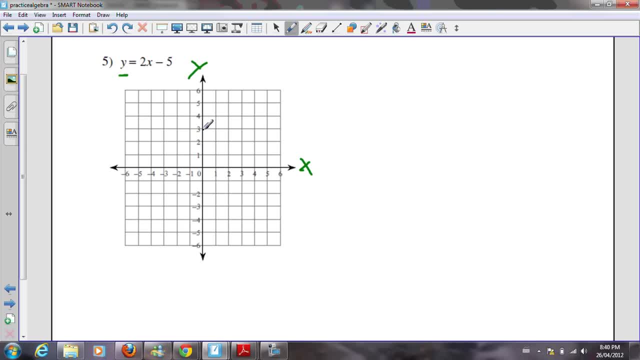 will end up being, say, 3, then you're going to end up with your y value of 3.. So you're going to end up with two things: You're going to have an x value separated by a comma and a y value. 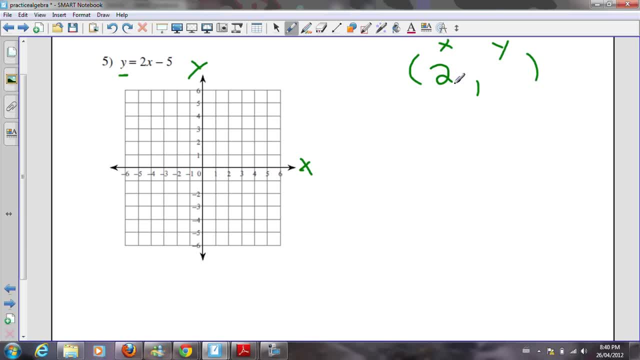 So I could start with x. Let's say x was 2. And I plug 2 into my formula here. So if I put 2 in for x, 2 times 2 is 4.. Take away 5 is going to leave me with negative. 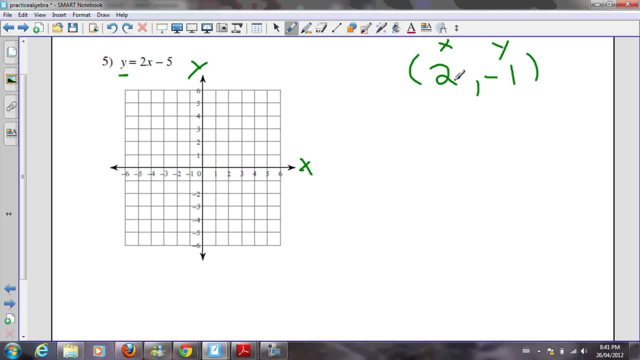 1 will be my answer. So I will plot this now And I'll start with my x. So you always start from the middle And you say, okay, x is positive 2.. So I go over 2. And y is negative 1.. 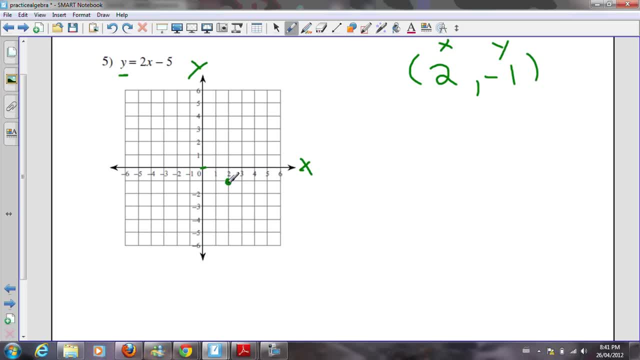 So I go down 1 to negative 1.. And there's my first point plotted right there. But how do you know which numbers to use? Generally, whenever you're given an equation and you're asked to graph it, the easiest way to do it is just simply. 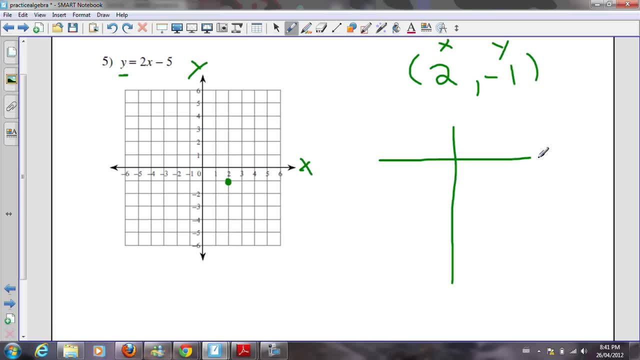 make your graph like this: Put x on one side and put y on the other. The x is your input or the numbers you're choosing, and the y will be your answer or your output. So we'll start with negative 2,. 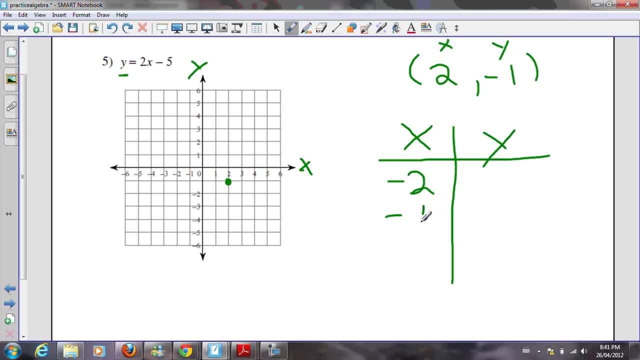 negative 1,, 0, and the y will be your answer or your output, And then we'll go with positive 1.. I'll put the plus sign there, although you don't really need it. You know it's positive. 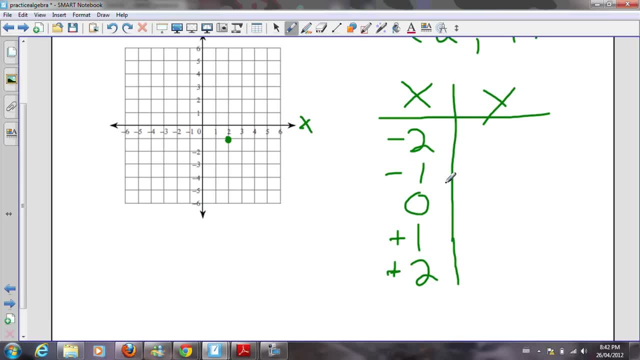 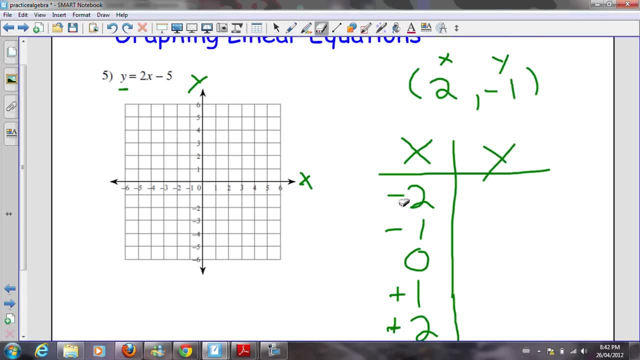 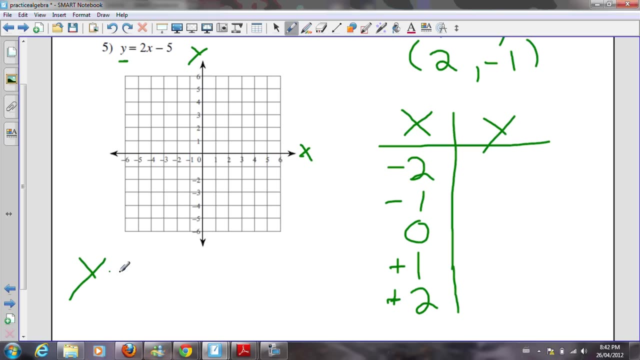 even if it was just written 1.. Usually we pick a couple numbers below 0, and a couple above, So let's start with the first one. Let's plug in negative 2 for x, So our equation, which is y equals 2x. 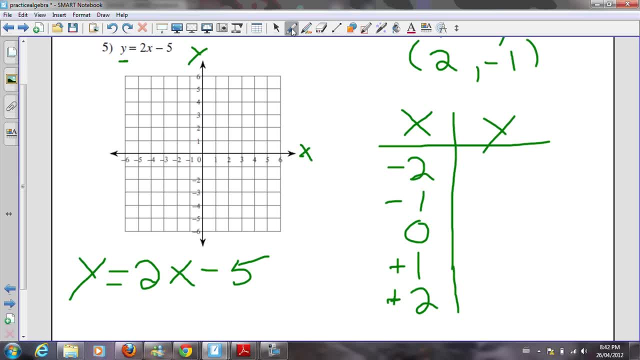 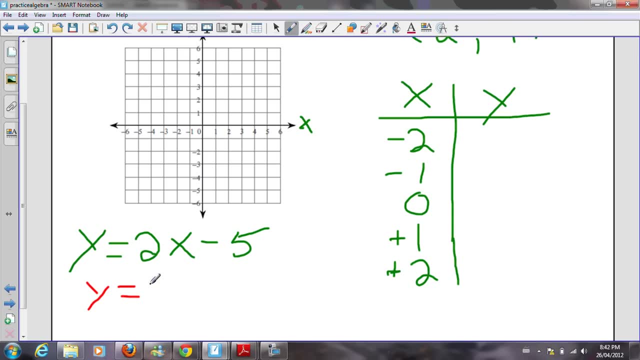 take away 5,. I'm going to plug in negative 2, because that's my first one. So let's do that: y equals 2 times negative 2, and then take away 5,, of course. Now let's keep going and keep solving. 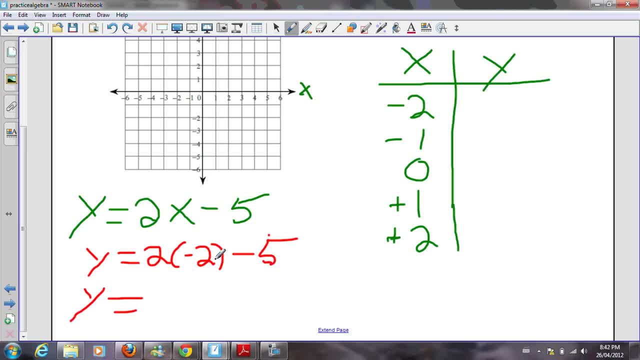 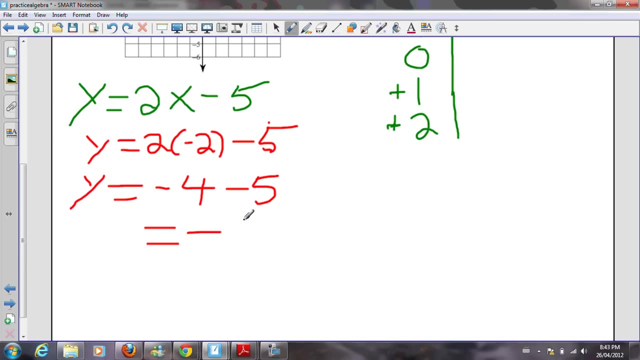 So y still equals. well, 2 times 2 is 4, but since it's a positive and a negative, it's negative 4.. Take away 5, so it's going to become even more negative. So negative 4. take away 5 equals negative 9.. 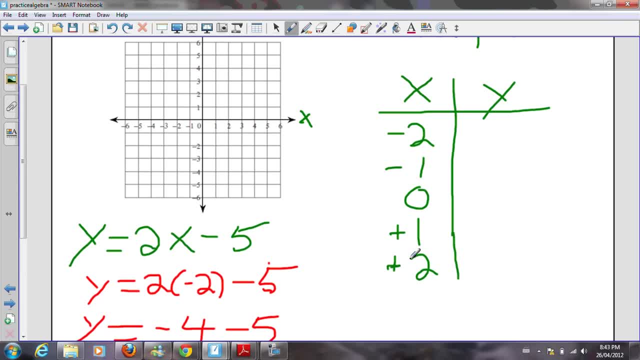 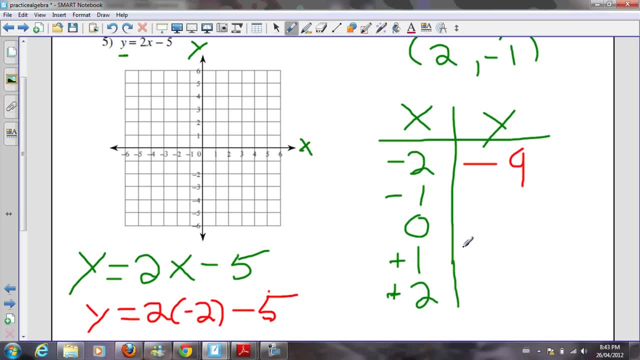 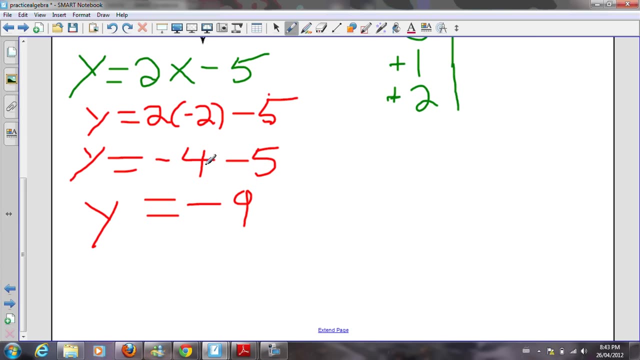 So our answer here is negative 9 for y. So when x equals negative 2, y equals negative 9.. Now let's try putting x in as negative 1.. So I'm going to go down, use the exact same equation. 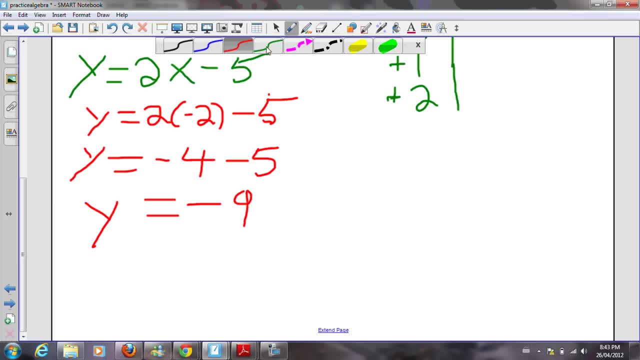 I'll rewrite it again down here. So remember our equation. It is: y equals 2x subtract 5.. Now of course I'll put in my negative 1.. So y equals 2 times negative 1, take away 5 more. 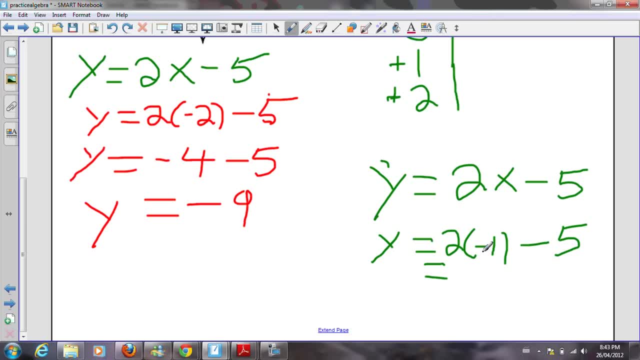 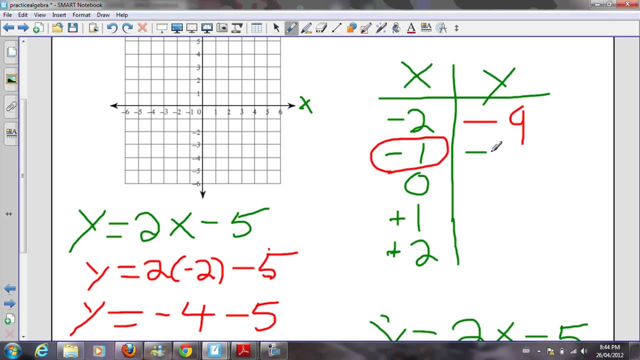 So 2 times 1 is 2.. Since it's a negative, it's going to be negative 2, take away 5 more and my answer for y is negative 7.. So when x is minus 1, y will be minus 7.. 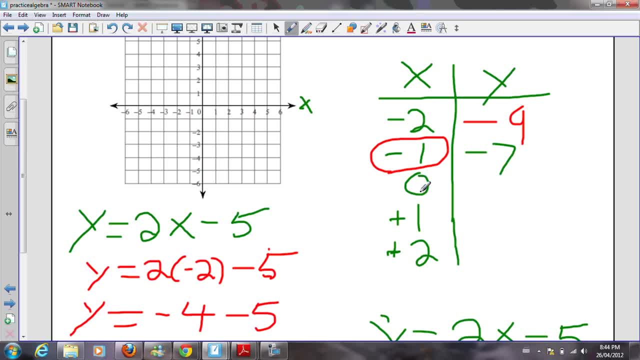 I'm going to do one more, because 0 is really easy to plug into any formula. If we put 0 into here for x, it's going to be 2 times 0. Well, 2 times nothing is still nothing. Take away 5 from nothing. 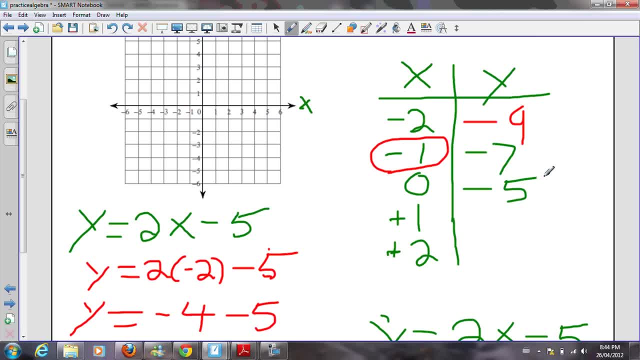 and we're going to be minus 5.. So you notice the pattern that's happening. You can look at your first one here is going up by 2, because it's becoming a little bit more positive or a little less negative. 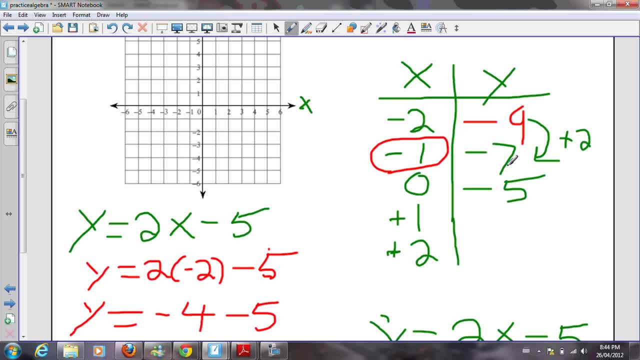 whatever way you want to look at it. So in this case it's going up by 2.. And again it's going up by 2 when you go from this one to this one. So really we could pretty much fill in the next two numbers. 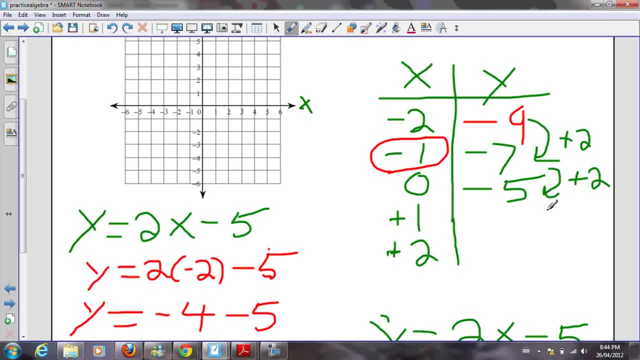 without having to work it out. So let's add 2 more onto minus 5, and that'll be minus 3.. And then the next one: when we add 2 more, it'll be minus 1.. So it's a little trick too. 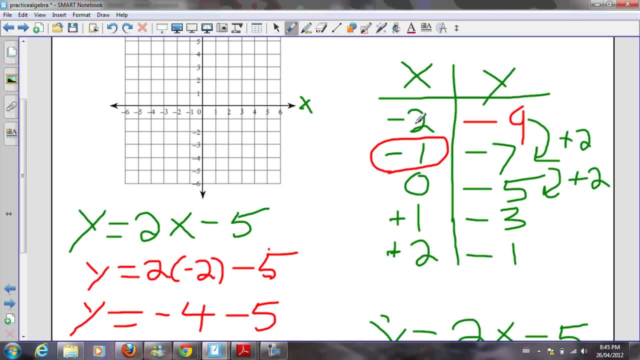 solving the rest of them. I like to do 3 numbers because you can see if you made an error in one of them. If you do 3 of them, you can really see, And if you get the pattern, the same. 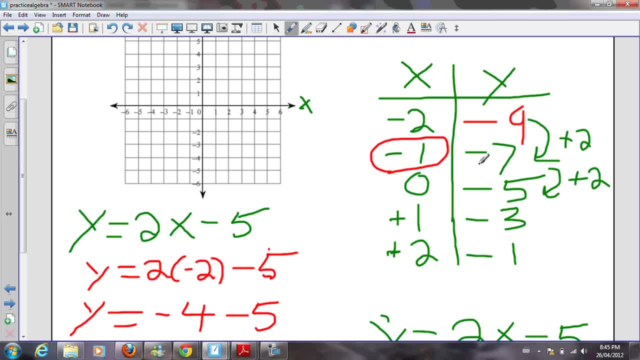 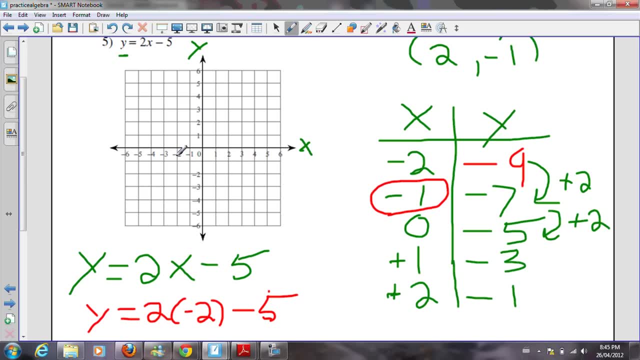 you know you're right. So there's our coordinates. So let's start with x at minus 1.. So x at minus 2.. So there's minus 2.. And y is minus 9.. And, of course, 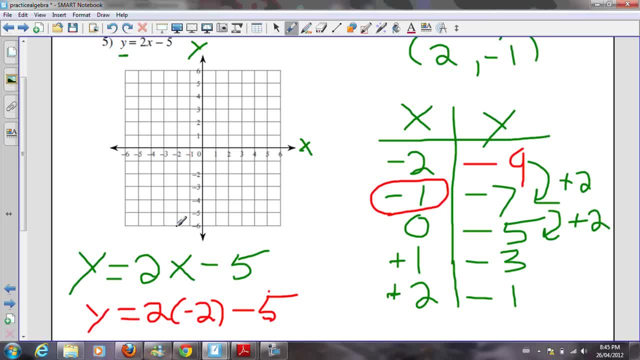 I don't have enough space here. I got minus 6.. So I'd have to go down 3 more. So that's minus 6, minus 7,, minus 8, minus 9.. So I'd put my dot right there. 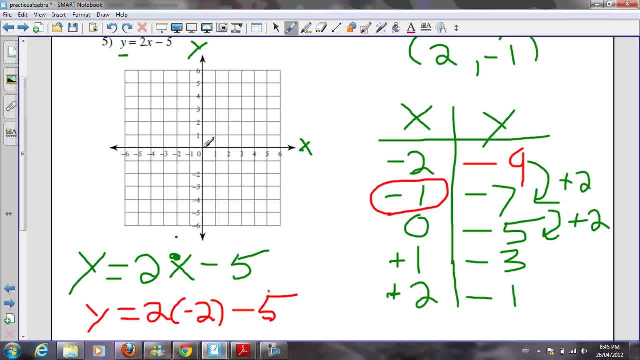 Let's do another one, Minus 1,, minus 7.. So we start there in the middle and go over negative 1 for x and go down negative 7 for y, Which'll be about right there. 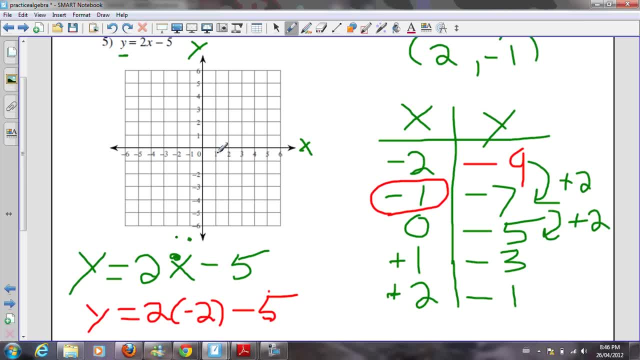 Again, your graph on a test will be complete or will have enough. Now I'm gonna put in 0, and negative 5.. So I'm starting at x. I'm gonna go over 0.. Well, that's easy for x. 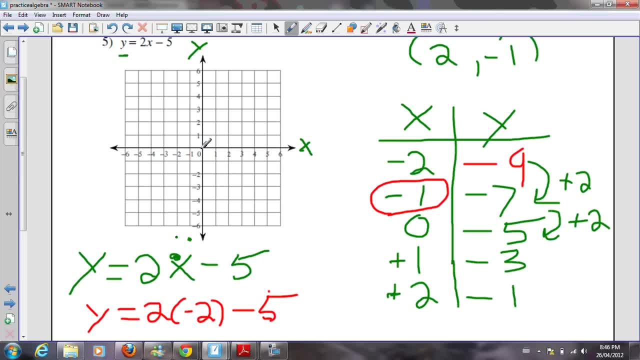 I just don't move And then I go down 5.. Because I'm going to negative 5.. I'll plot another one. It's gonna be positive 1, and negative 3. So I'm gonna go over positive 1,. 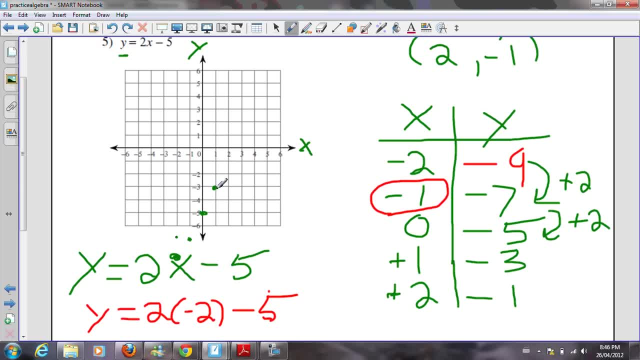 and down: negative 3. And finally, positive 2.. So I'm gonna go over 2, and then I'm gonna go down 1.. And, as you can see, if I were to draw a straight line, providing I had done this- 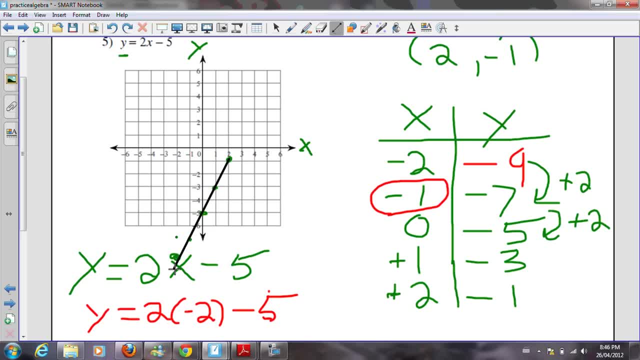 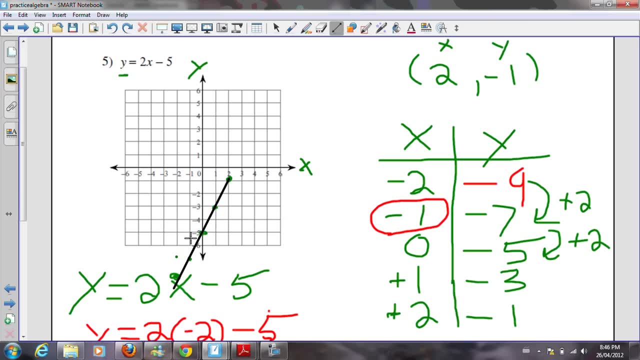 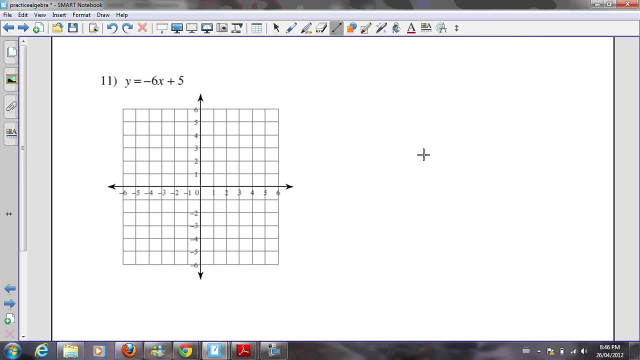 pretty accurately. you notice, all of it should be in a straight line, Because this is a formula for a a line. So if it's not all in a straight line, you also know that your answer must have been wrong. Let's try one more. 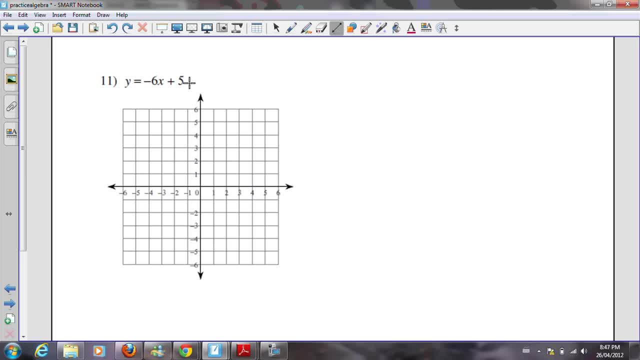 Here we have negative 6x plus 5.. For this one you again draw your table like this: You put in your x on one side and your y on the other, And then you give your minus 2,. 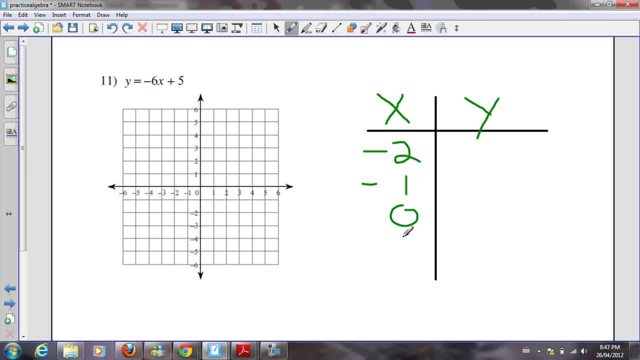 minus 1, and 0.. 1 and 2.. Now do we have to pick those 5 numbers? It's not totally. you could have picked 1, 2,, 3,, 4,, 5.. But you do have to make sure. 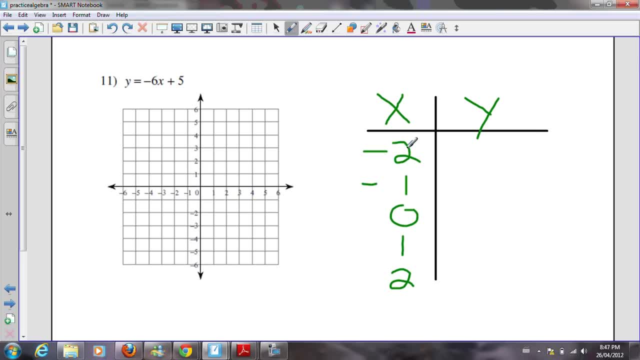 that all the numbers are in order. In this case, they're going up by 1.. So if you had to pick 1, 2,, 3,, 4, 5, it'll still work. So the only thing you have left to do. 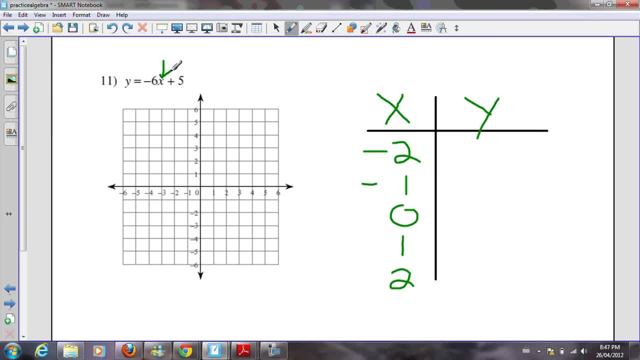 is plug in minus 2, into your equation right here for x, And then see what you get. So if I put minus 2 in here, it's going to be negative 2, times negative 6,, which is positive 12,. 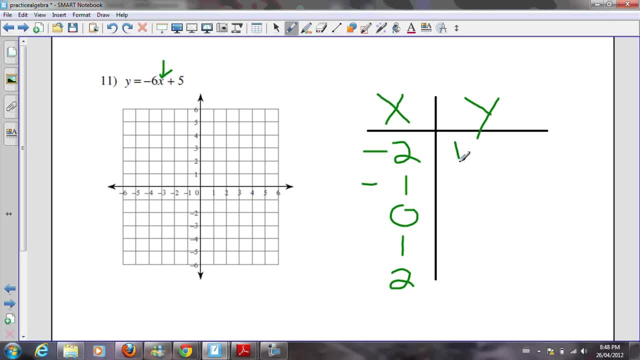 plus 5 more is positive 17.. Now, right away you can see there's no way to graph it on this. You would need some graph paper and you would have to make your own coordinate grid. because negative 2,. 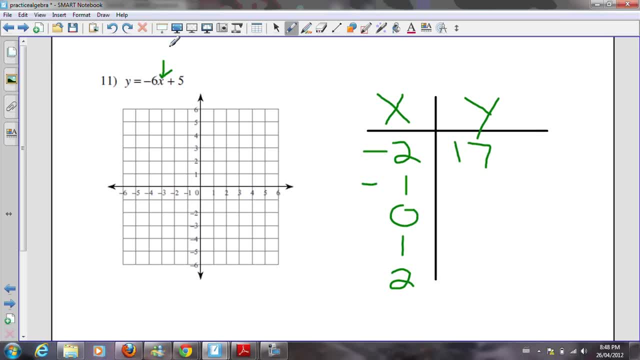 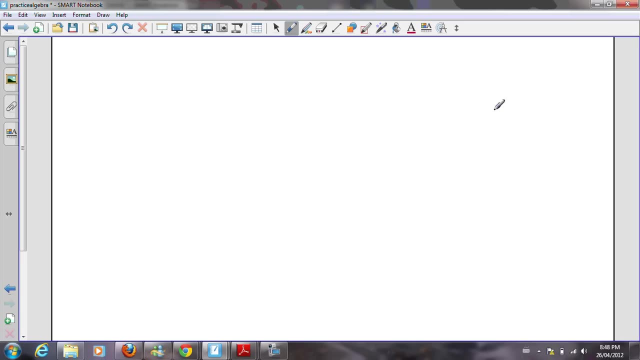 and positive 17, would be way up here somewhere. Okay, So that's not a very good numbers to choose these ones right here. The ones you will be given, of course, will be much easier to choose from, and you just go ahead and draw your. 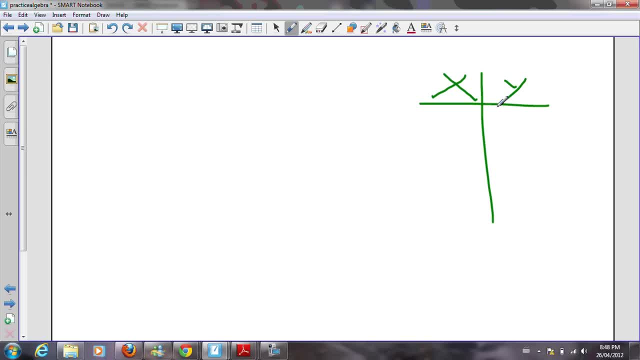 table with x and y each time And then put your numbers there and just plug them in, and once you get three of them done, you don't really have to do the rest. You can just see the pattern that's going up here. 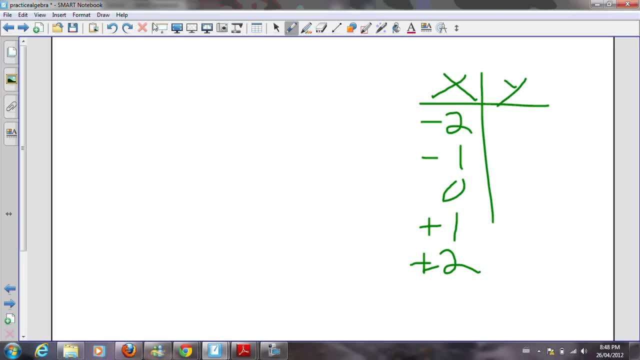 and keep jumping like that. So I hope this has been helpful for you and if there are any questions or any problems and you need some help with it, feel free to email me at MrEdison at hotmailcom. 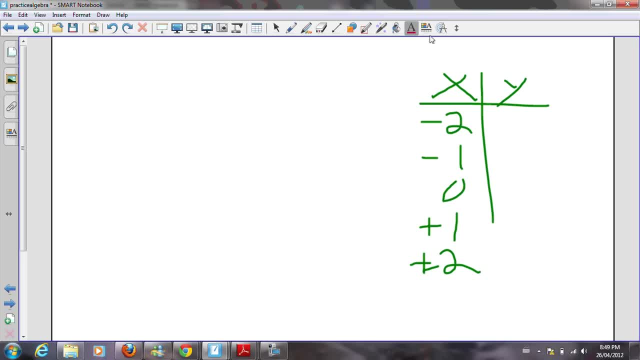 and of course nothing's coming out on the computer, so I'll put it here. So it'll be, MrEdison. my goodness shocking. I'll try that one more time. Okay, so MrEdison at hotmailcom.